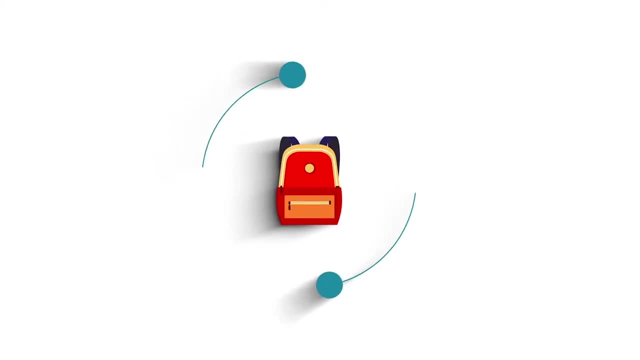 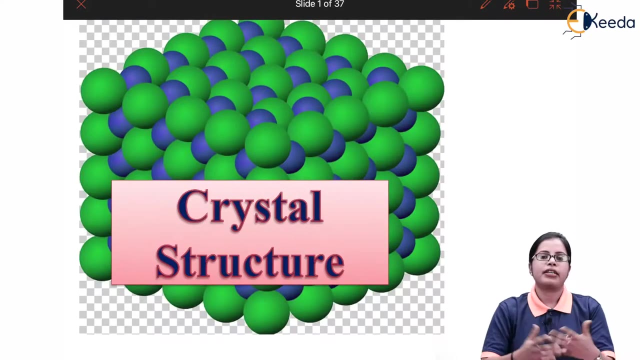 calculation of crystal structure. Once we are starting with the concept of crystal structure, the concept comes from like: when we talk about matter, matter is divided into three parts, that is, solid, liquid and gases. But we are specifically talking about only solids. When we say solids, 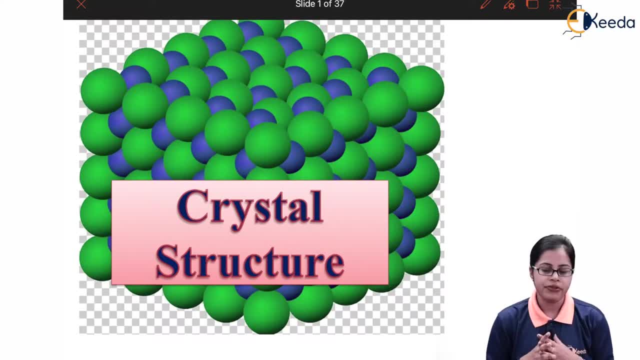 solids consist of atoms or a group of atoms together which are arranged in very close proximity. That is why they are considered to be solid. But when we talk about the physical properties of the solid or the physical properties of the solid, or the physical properties of the solid or the physical, 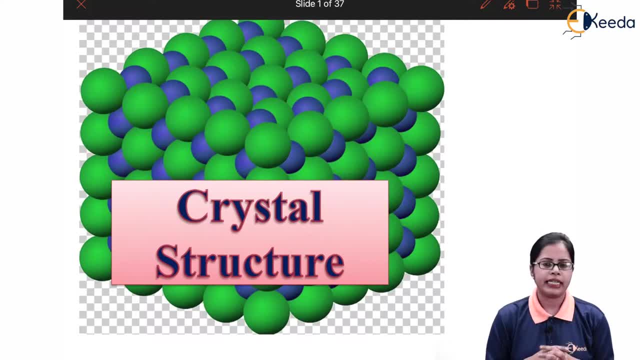 structure of the solid or the normal properties of the solid. everything is entirely dependent on the arrangement of the atoms inside the solid. So we can say that the structure of atom, or you can say the structure of material structure of any solid and the properties of the solid is 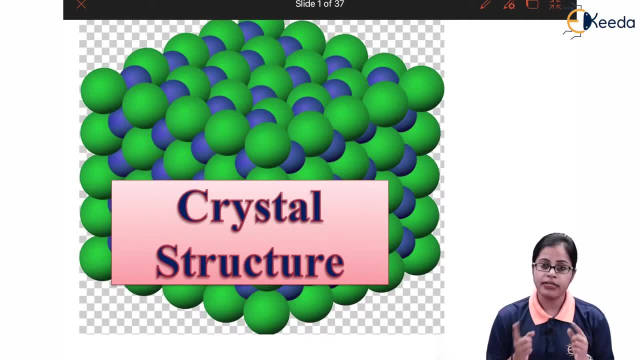 entirely dependent on arrangement of the atoms inside the solid. Now we can have two types of arrangement. Either I can have random arrangement or I can either have proper ordered arrangement giving me different classification of the materials. So when we talk about this classification of materials, it can be classified into two types. 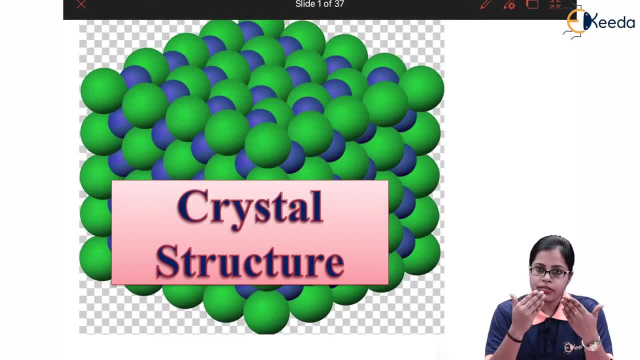 basically dependent on arrangement of the atoms inside the material, firstly. Secondly, we are going to make use of certain basic geometrical concepts, such as lattice or unit cells, So has to describe the arrangement of atoms, and such as to formation of crystal structure. So these geometrical concepts are very much important in terms of 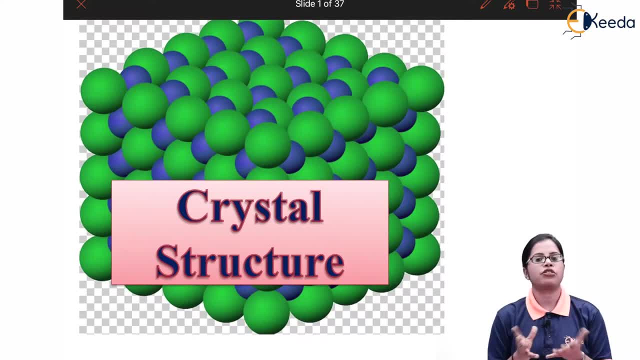 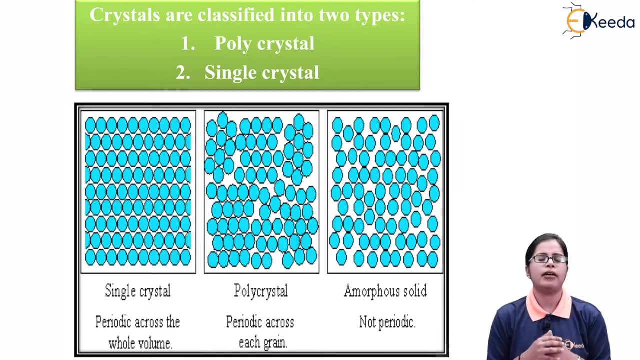 if we want to get to know that, how is crystal structure getting formed? we should be aware of the geometrical concepts. So when you say about the classification of material, I said the materials can be classified basically into two types. So we can have two types of arrangement of atoms inside the solid or 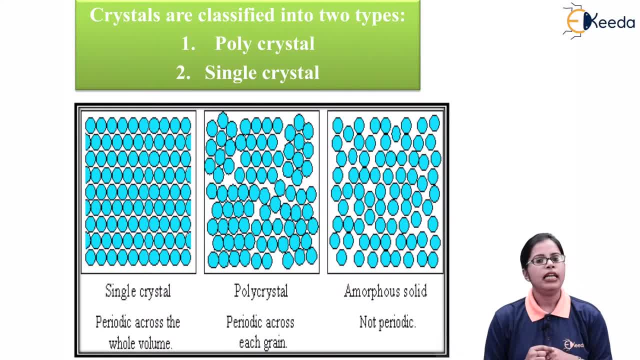 on the arrangement of atoms inside the material, Like if the material consists of ordered arrangement of atoms, it is going to be considered as crystalline material. But if the arrangement of atoms is entirely random or the arrangement is considered to be of a random orientation. 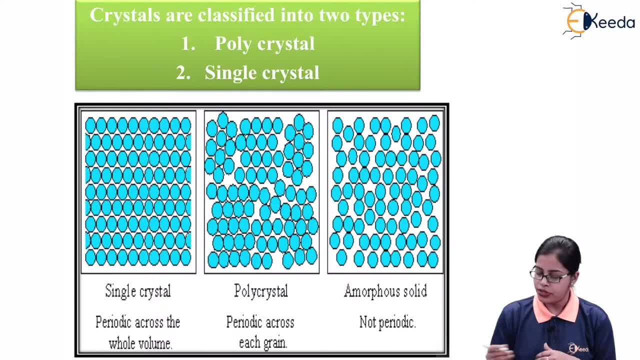 in that case the material is classified as amorphous. So either I can have material which is crystalline and the second type is the arrangement of atoms inside the material. So the second type of material that is basically dependent on arrangement of material or arrangement. 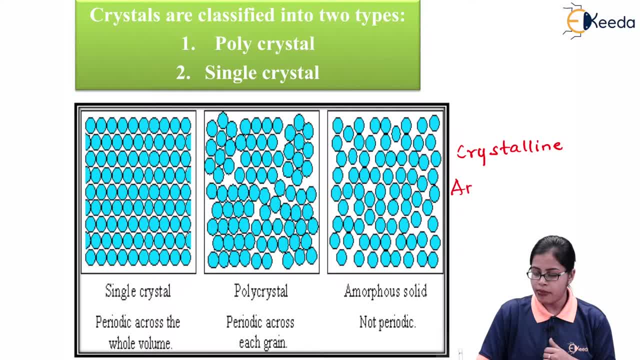 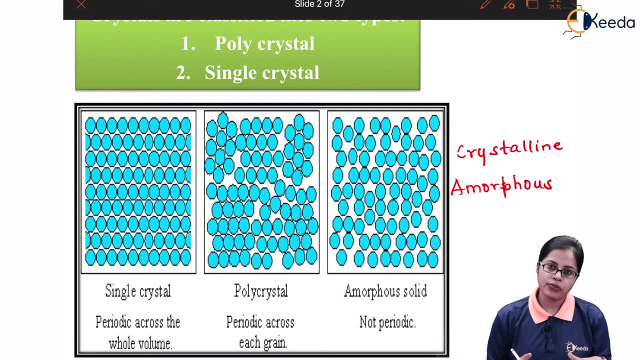 of atoms. it is going to be classified as amorphous. So we have materials classified into two types: crystalline and amorphous. Now, when you talk about the basic concepts like ordered arrangement is going to give me crystalline material. amorphous means random. 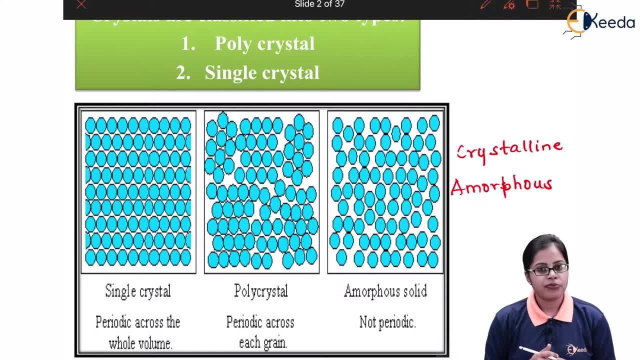 orientation of atoms is going to give me crystalline material. So if I have a material, is going to give me amorphous material. when you talk about crystalline, or specifically the crystalline material, crystalline material is classified into two more types that are: 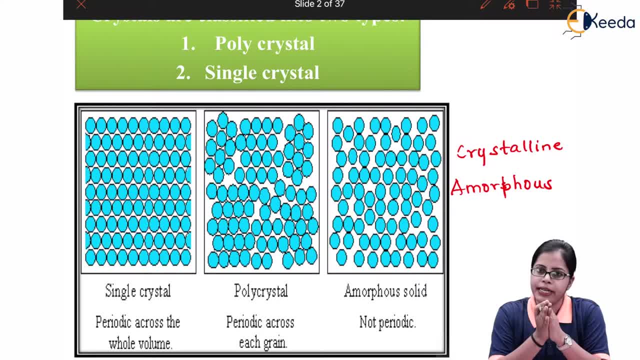 single crystal and polycrystal. Now, what do you mean by single crystal and polycrystal? is that if we have ordered arrangement of atoms throughout the entire volume of the crystal, that means or particular proper arrangement of atoms inside the material. 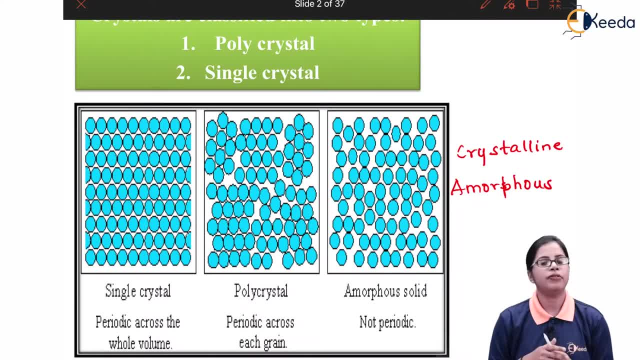 in that case the crystalline material is considered to be single crystal. But when you talk about polycrystalline, in polycrystalline we do not have ordered arrangement. throughout the volume It consists of fine grains which are separated by each other with the help. 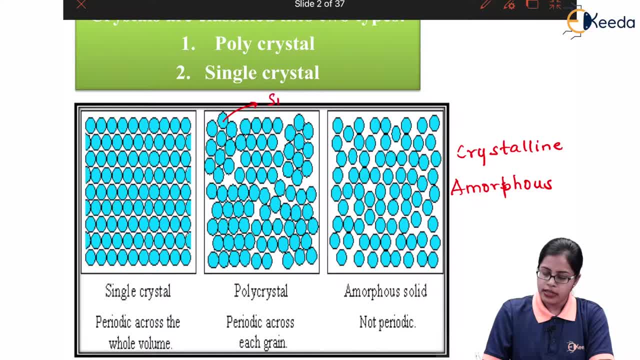 of boundaries And this grains of the polycrystal material are in the range of a single crystal. in that case it is considered to be single crystal And this grains of the polycrystal material are in the range of one single crystal. So that is the order of the volume of the 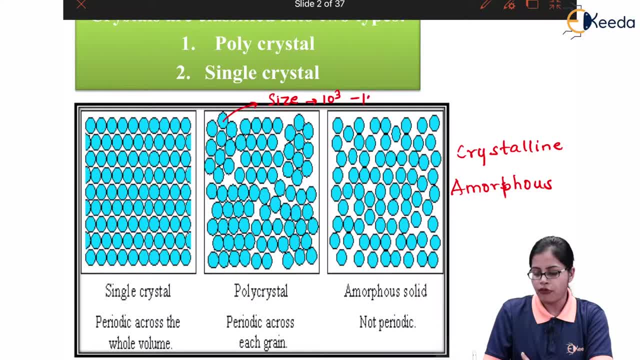 of size that is, from 10 raised to 3 to 10 raised to 4, Armstrong. So if we consider polycrystalline material, it is going to consist of fine grains, which is of size 10 raised to 3 to 10 raised to. 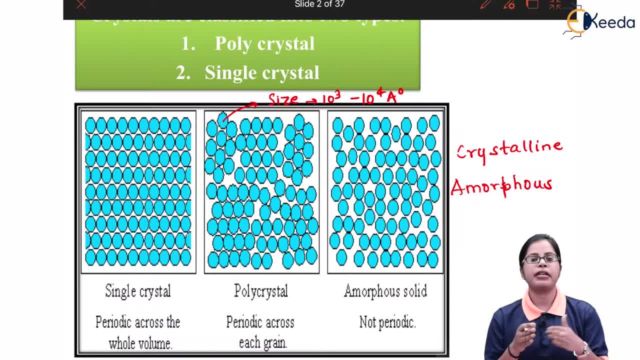 4 Armstrong, and they are divided or they are separated by well-defined boundaries. and when you look at the whole orientation, the boundaries and the fine grains, they are going to have different orientation with respect to each other. But if you look at the grains which are arranged, 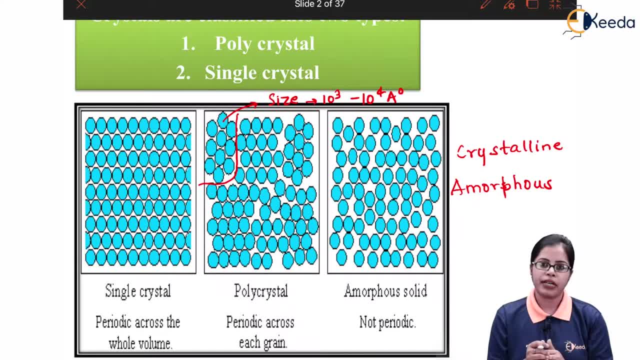 in one boundary they are oriented in one particular direction or they have ordered orientation. But if I compare it with some other boundary it is going to have random orientation or different orientation. that means what they do not have: ordered arrangement throughout the volume. they have order in arrangement in a particular grain. 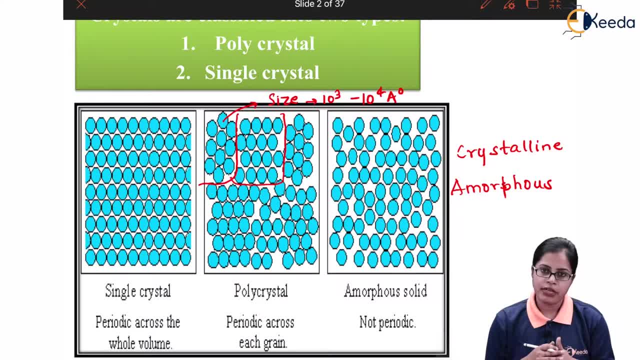 So if we consider polycrystalline material, that means we can have crystalline material and amorphous, and crystalline can be further classified as single crystal and the polycrystal. When you say single crystal, the order arrangement of atoms throughout the material is going to be: 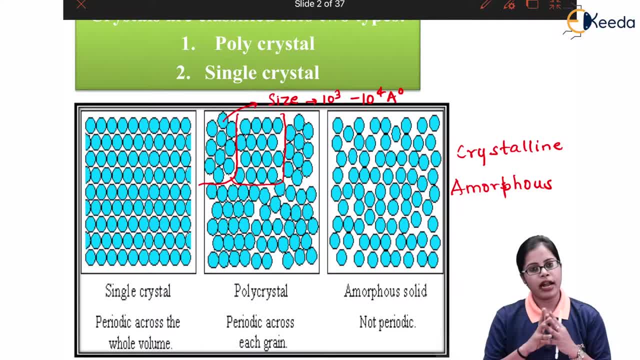 considered as single crystal. But if you have random orientation of atoms throughout the material or you can say you have any different orientation of atoms throughout the material, you can say you have any different direction orientation, that is considered to be amorphous. But when you talk about single crystalline and polycrystalline, entire volume has a orderness. 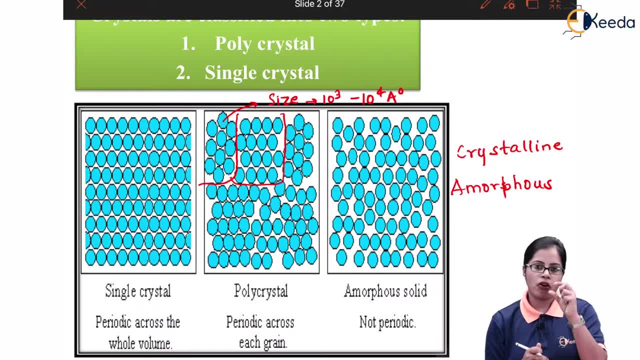 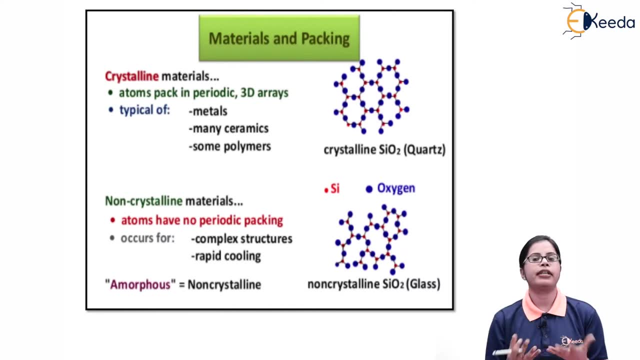 it is going to be single crystal. But if you have orderness in a certain boundary or in a fine grain format, it is going to be called as polycrystalline. So that means when you say orderness we can even name it as periodic across the whole volume or the periodic arrangement. 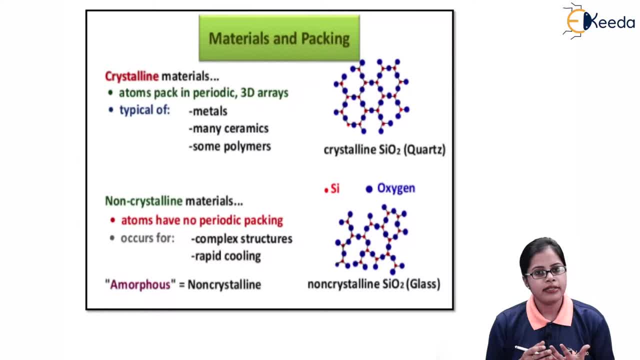 of the atoms. When you say materials which are made up of either crystalline nature or materials having amorphous nature, So some materials are going to have a crystalline nature and some materials are going to have amorphous nature. When you say atoms are packed, completely, packed in periodic. 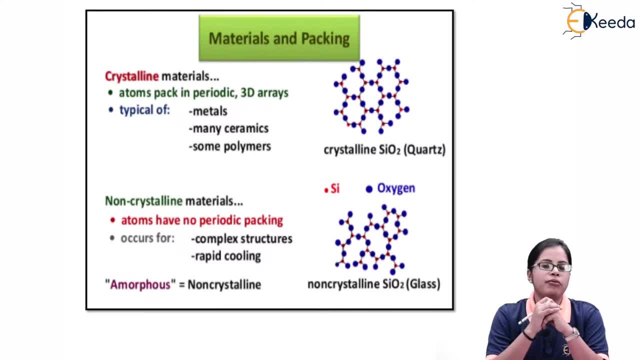 arrangement in a 3D array that is going to be considered as crystalline material And the basic idea of crystalline material is considered to be metal. Many ceramics are considered or classified under crystalline material. Some polymers are even considered to be crystalline. 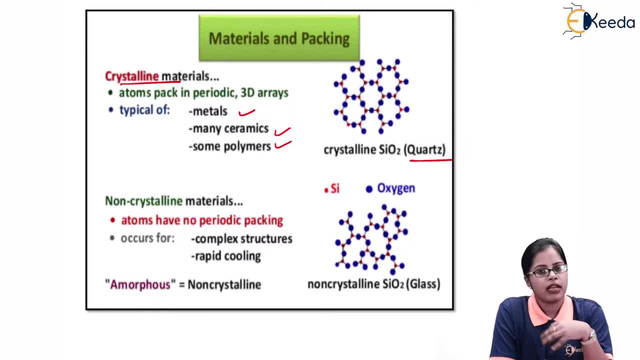 in nature. For example- I have given over here as quartz. Quartz is considered to be crystalline in nature, but if I have a non periodic arrangement of atoms in a certain 3D packing or something, in that case that particular material is going to have a amorphous. 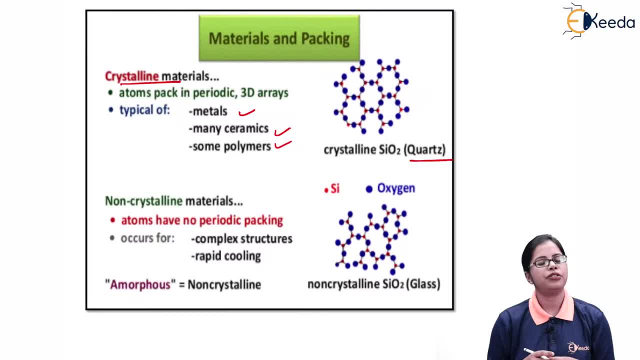 nature. And second thing, because of the random orientation of the atoms, the structure of the amorphous material is very complex and they are considered to have a very rapid cooling, or super cooled solids or liquids. Secondly, when you talk about the non-crystalline, you can take an 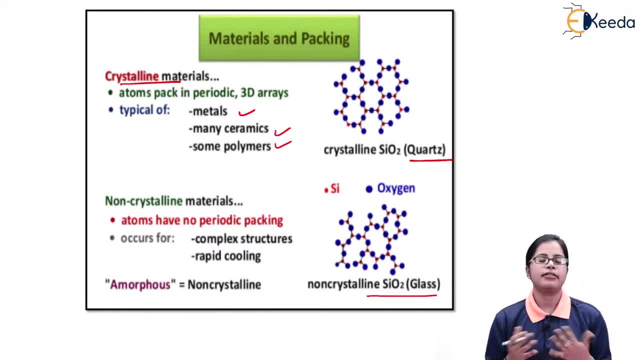 example of glass, which is a daily life example. Glass is considered to be amorphous in nature and when you say non-crystalline, it is just another word for amorphous. So non-crystalline is considered to be amorphous. Next is: this: is how you classify the material into two. 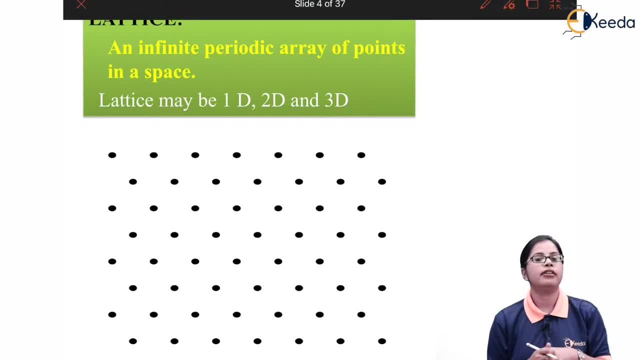 different parts, either crystalline nature or either amorphous nature. But when you talk about the concepts of crystal, we need to consider certain geometrical concepts. that is, lattice unit, cell bases. These are all important geometrical concepts which we make use of while formation of crystal structure. So we need to consider certain geometrical 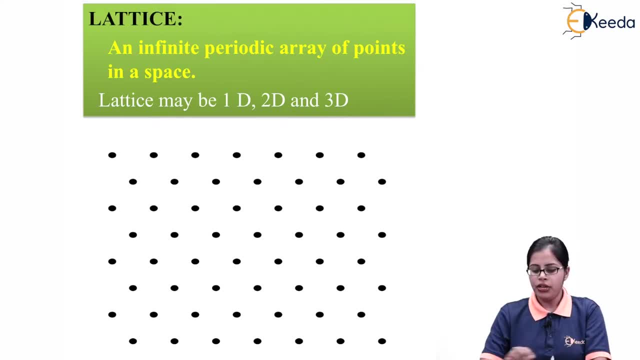 concepts, that is, lattice, unit, cell bases. These are all important geometrical concepts which we make use of while formation of crystal structure. Now, when you talk about lattice, what do you mean by lattice? We consider this lattice as an imaginary concept entirely. 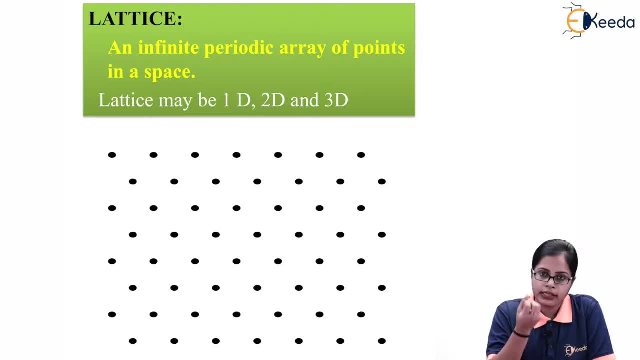 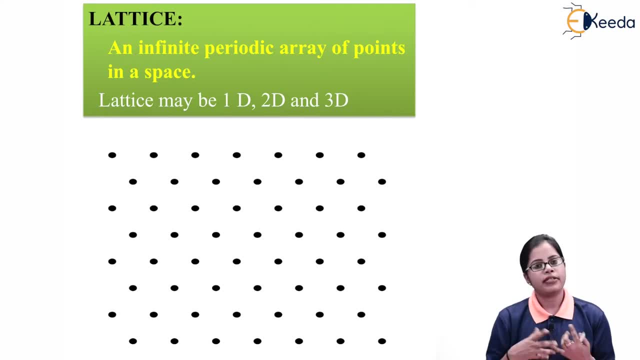 in 3D array, then we can say that this is a 3D array. So that means if we consider an infinite dimensions, So like, simply, if it is asked, what do you mean by latice? Latice is nothing but. 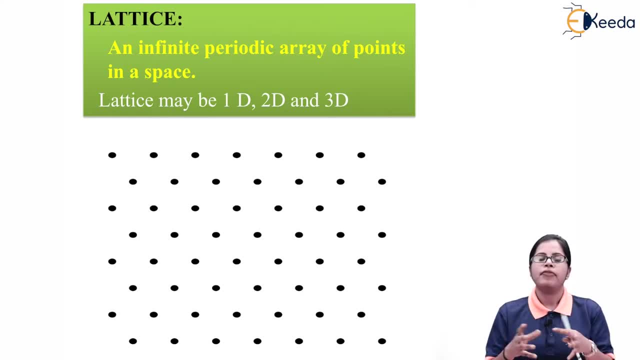 an array of infinite number of points which are arranged in one dimension, two dimension and three dimension. But most commonly we make use of three dimension because all the structures are considered to be in three dimensions. So we can just keep in mind that latice is the periodic arrangement. 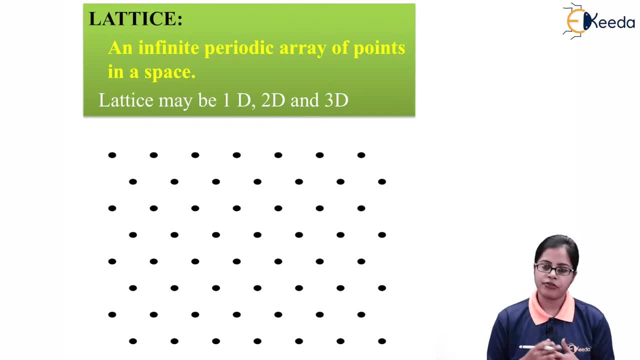 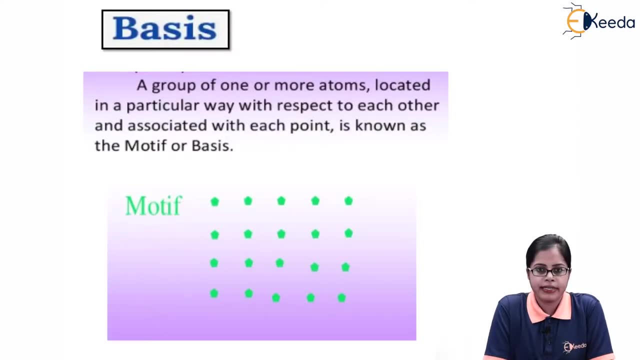 of infinite number of points. that is what is going to lead to the concept of formation of crystal structure. So next is when you say basis. basis is something as you can consider, a group of one or more atoms which are located in a certain manner, Like 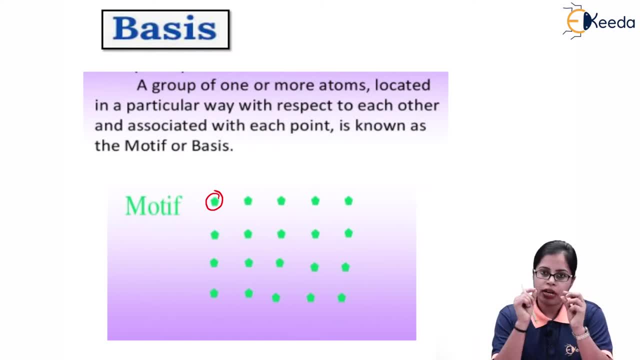 if I consider a certain group of atom located at a particular position, I can again consider a certain group of atoms located at a certain distance from the previous group, As in this manner I can arrange a large number of group of atoms together, but in a periodic arrangement. 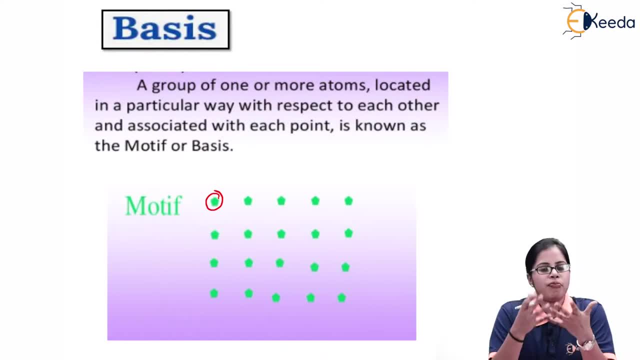 not in a random arrangement. So if we have a group of one or more atoms which are located in a particular way, obviously with respect to each other, Now this group of atoms are nothing but called as basis, Like if I consider this has a group of atom which is located at a certain 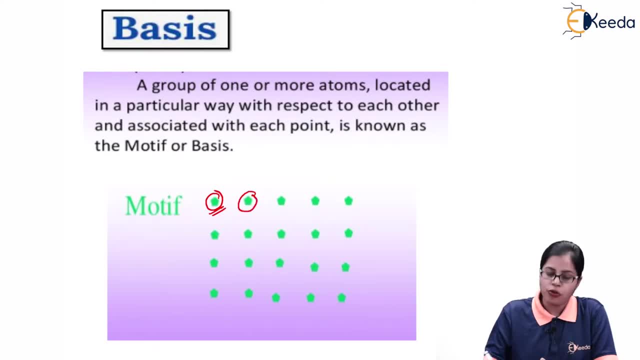 position. I have again certain group of atoms which are located at a particular position. Normal group of atom is a group of atoms located at a different position and also a group of atoms located at same orientation. Normal group of atoms is like written Ground treatment. 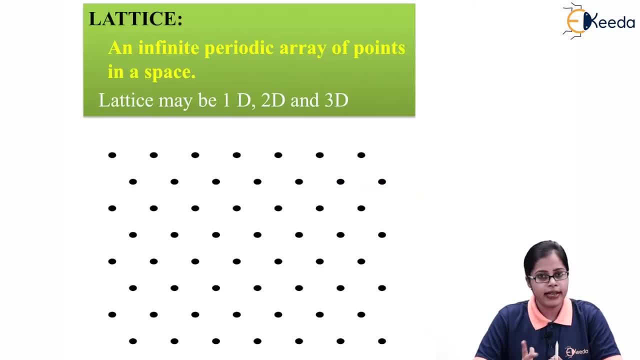 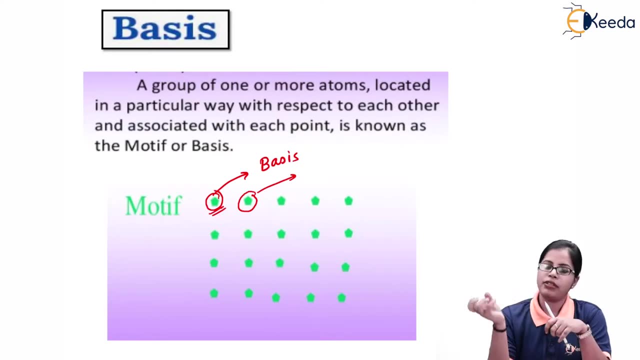 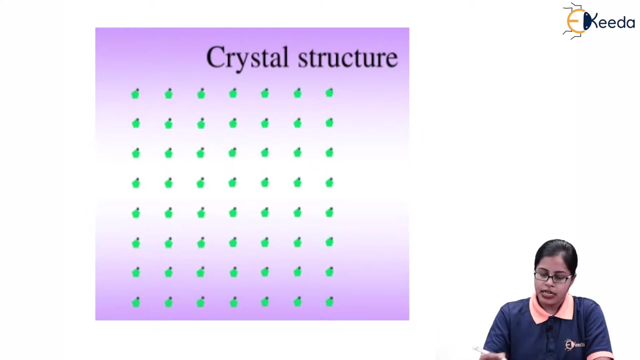 now, what are we going to do with these two things, that is, lattice and basis? we are going to associate each basis with each lattice. that means we are going to attach basis with lattice so that whenever I attach basis with the lattice, it is going to give me the formation of crystal structure. 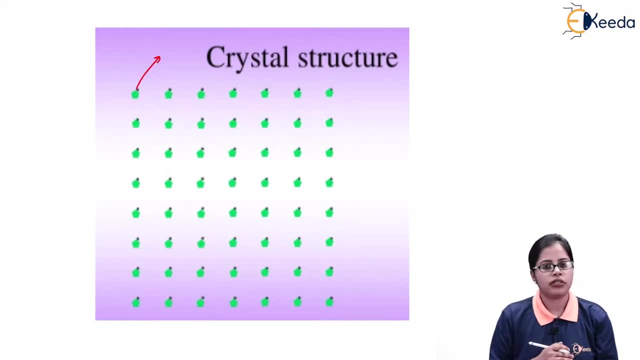 so those black points, or the black dots, are indicating the lattice point and, as you can see in the diagram, I have a periodic, infinite number of points which are arranged in a 3d array, and those green circles are indicating nothing but the group of atoms which are nothing but called as basis. so what I have done is I have attached basis with 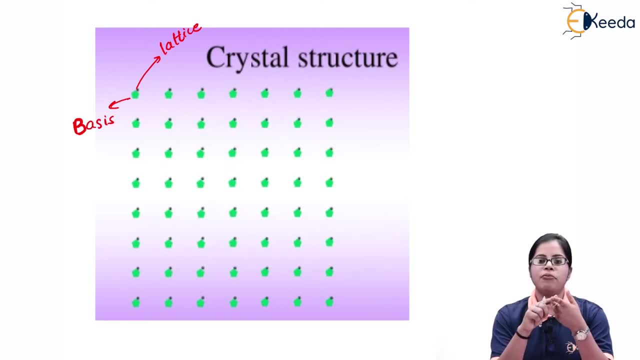 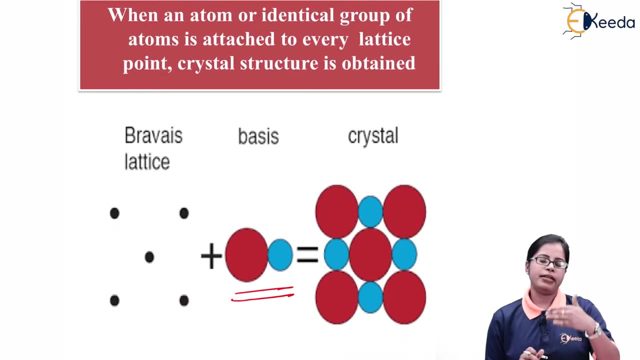 lattice. So and the basis with lattice combination is going to give me the formation of crystal structure. So, whenever we want to form basis with crystal structure, we need to attach atom or identical group of atoms to every lattice point. and whenever we are doing this process of attaching atoms or 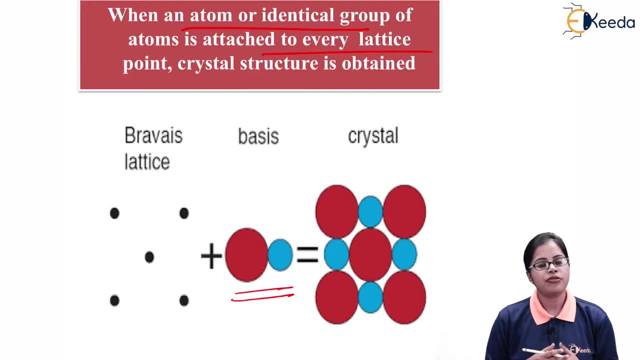 group of atoms to every lattice point. that leads to the formation of crystal structure. Next is, as you can see in the diagram, that we have this points to be the lattice and this to behave as the basis. So if we take or if we attach this basis to each and every lattice, it is going to lead to the formation. 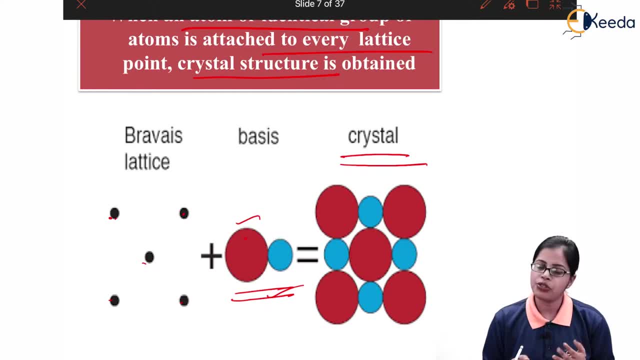 of crystal. That means a simple combination of bases attached to each and every lattice point is going to lead to the formation of crystal structure. So that is why I said that some geometrical concepts like lattice basis are most important to get the information that how is the crystal structure? 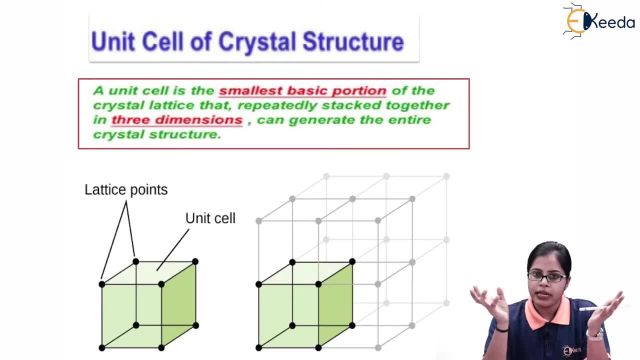 being formed. So just simply keep in mind that if you want to form a crystal structure, we have to attach each group of atoms to each lattice point. that leads to the formation of crystal structure. Next is, when we talk about crystal structure, there is something called as: 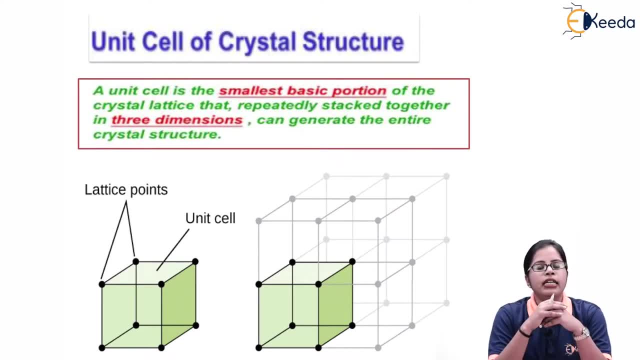 unit cell. Now, what do you mean by unit cell Before that, like we have done this from our school sections- that every material has a basic unit or a basic building block, and that basic building block is nothing but atom. So atoms behave as the basic building block or the basis. 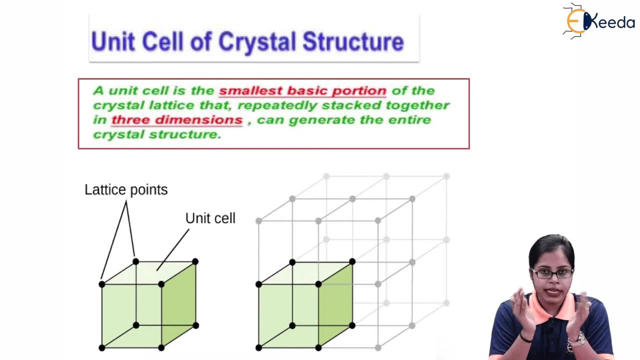 of The whole material In a similar manner, if I consider a unit cell, like for a crystal structure, the unit cell is the smallest basic portion of the whole crystal structure. So if I want to consider a unit cell, if I keep on stacking this unit cells together, then it is going to lead me. 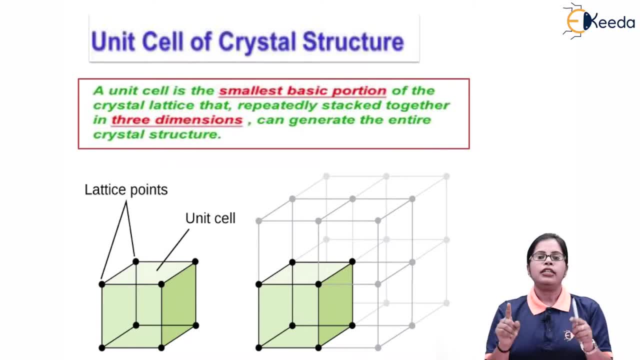 to the formation of crystal structure. That means what The whole crystal structure has a smallest structure. So if I keep on stacking this unit cells together, then it is going to lead me to the formation of crystal structure. That means what The whole crystal structure has a smallest. 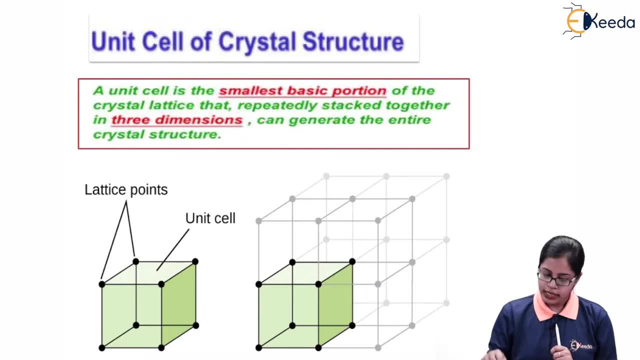 basic portion and that basic portion is called as the unit cell. That means you can say this, as the smallest basic or building block of any crystal structure is going to be called as unit cell. Now if you look at the diagram, this first diagram is indicating the diagram of unit cell. 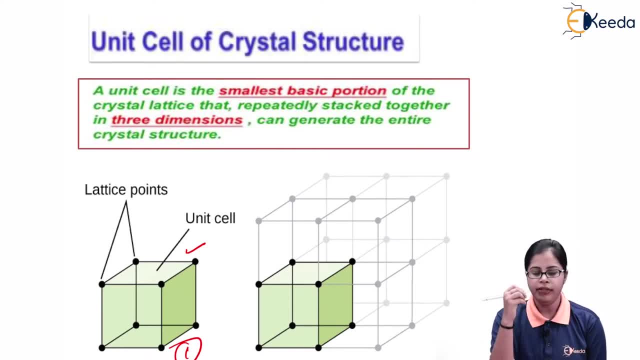 That means this is one block of unit cell which is considered to be of cuboidal shape. So I can say it is a cubic unit cell and this one unit cell is going to behave as the smallest basic portion, or you can say the basic building block, of the whole crystal structure. 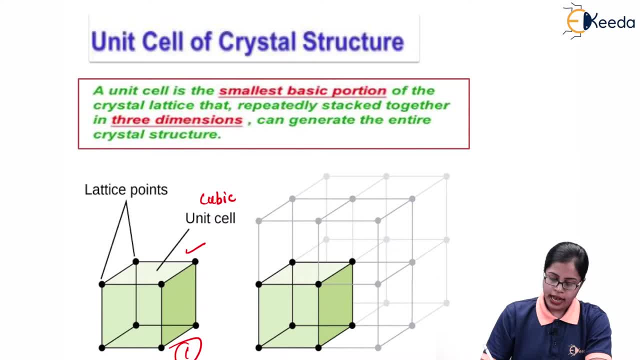 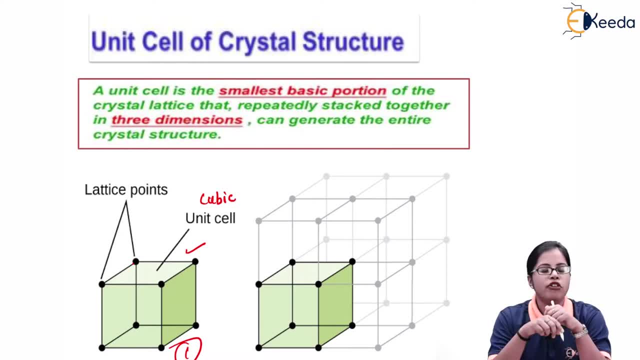 lattice points attached to the eight corners of the cubic unit cell. That means what? There are eight points attached to the eight corners of cubic unit cell. second thing: the line which is joining this two lattice point, that is, the lattice points at the corners, are joined by this line. so this line is called as lattice line. that. 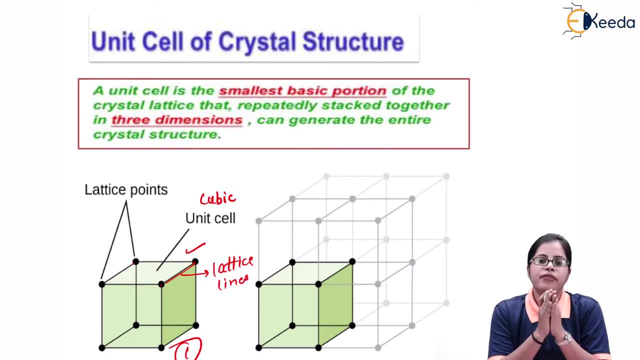 means at all the eight corners of unit cell. we are going to have the arrangement of lattice points, and the line used to join the lattice points are nothing but termed as lattice lines. now, as you can see, this whole diagram is indicating the 3d shape of crystal structure, but the basic building block 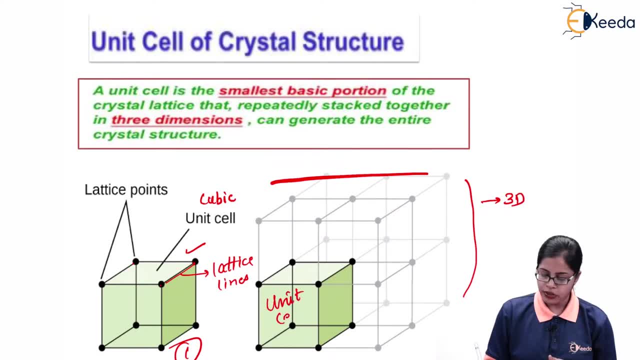 of this crystal structure is nothing but the unit cell. I have to stack many unit cells together to form the crystal structure. when you say basic building block, so unit cell stacked together is going to lead to the formation of crystal structure. so that means during the formation of crystal structure the unit cell is very much important. because if 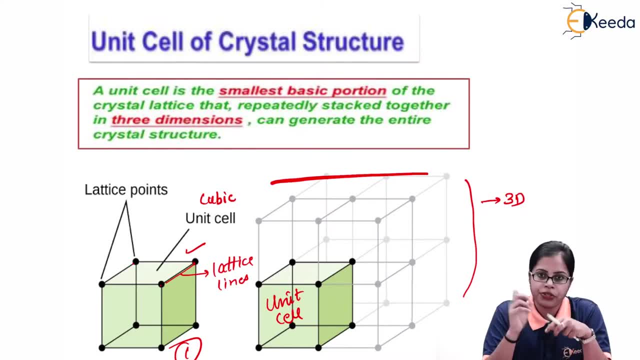 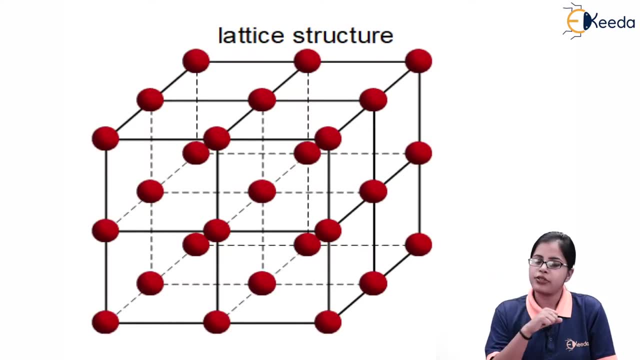 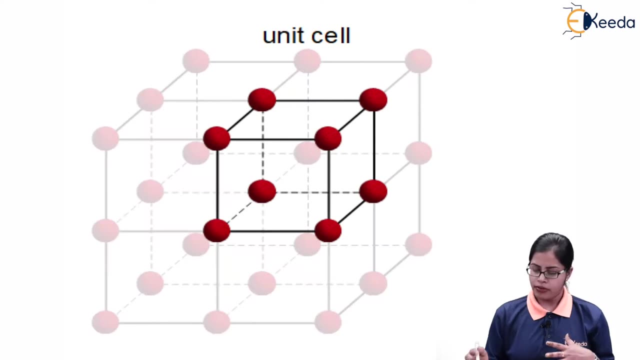 you are not making use of unit cell, you won't get the formation of crystal structure. now, as I said, for any crystal structure the basic building block is going to be unit cell. in this diagram I have shown it anemotically that when you talk about the unit cell, this is one unit cell having the eight lattice. 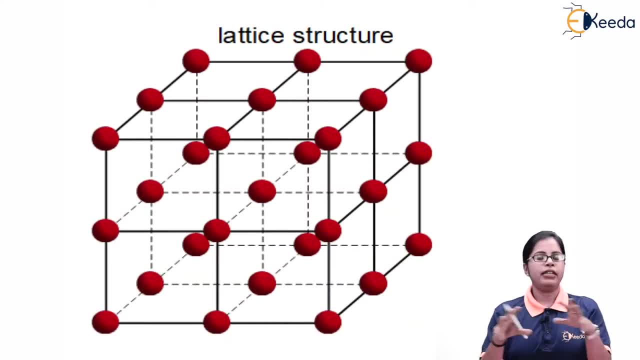 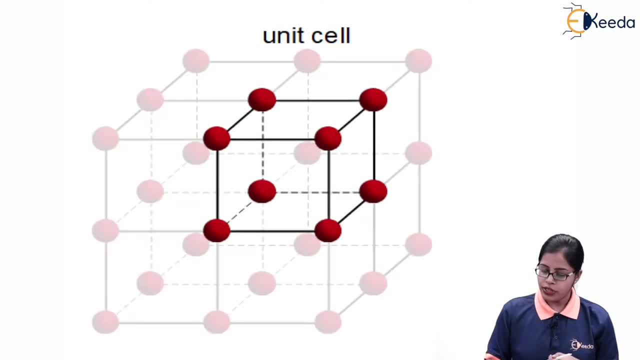 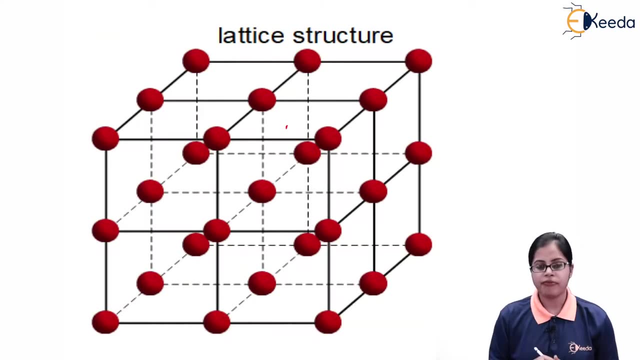 points and when I keep on stacking many more unit cells together, it leads to the formation of lattice structure, the crystal structure. so the first one is indicating this is indicating the unit cell and once you stack all together it is going to give me the lattice structure. so once we get to know how to 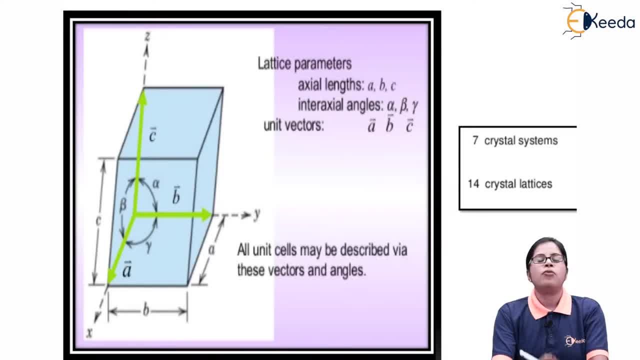 form a lattice structure. the next concept comes is: as we are aware of the formation of crystal structure, we are going to make use of the different lattice parameters which are used for the calculation during the formation of crystal structure. so the basic lattice parameters which we are going to make, 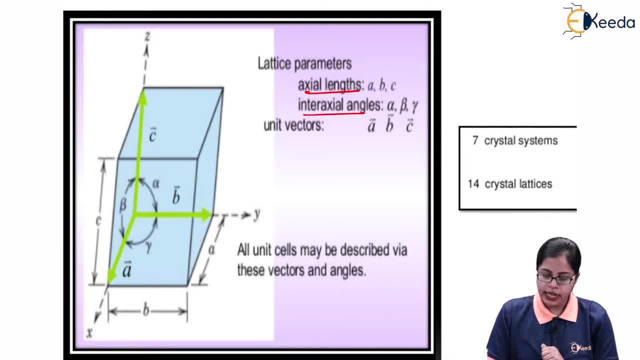 use of our axial length, interaxial angles and unit vectors. these are three basic parameters which we are going to use throughout this formation of the crystal structure. now this whole diagram is for unit cell and I have considered one corner of the unit cell to be behaving as an origin of a Cartesian 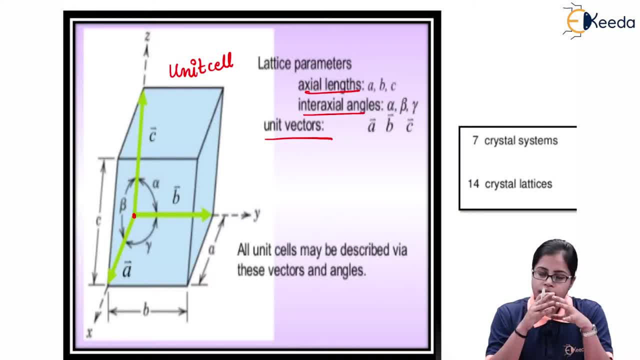 coordinate system and, as the diagram is moving in a 3d shape, or the crystal structure is in a 3d shape or the unit cell is in a 3d shape, so I have to consider three coordinate axes, that is, X, Y and Z. I've considered that this is x-axis, this one is the y-axis and this is 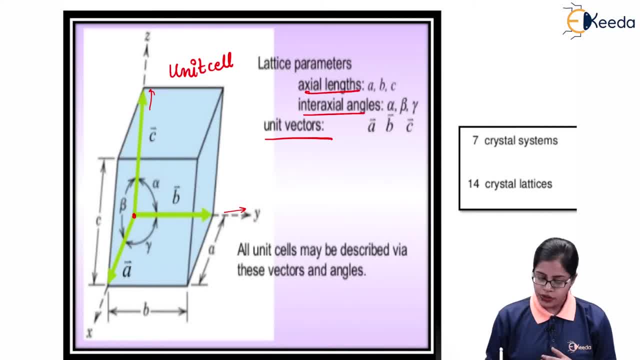 considered to be z-axis. second thing: the unit vectors, respectively along the three axis, that is, X, Y and Z, are considered to b vector, b vector and c vector. so this a vector is considered as the unit vector along x axis, and when we talk about b vector, it is a unit vector. 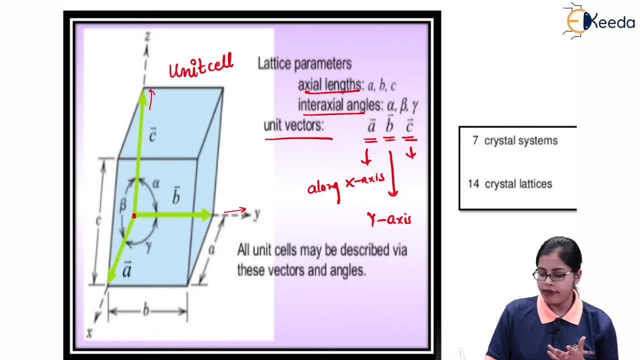 along along the y axis and when we consider c vector, it is a unit vector along z axis. Next is when you talk about the angles. as you can see, there is an angle separation between the two axis, like either I talk about the angular separation between the x axis and the y axis, or between y and z, or between 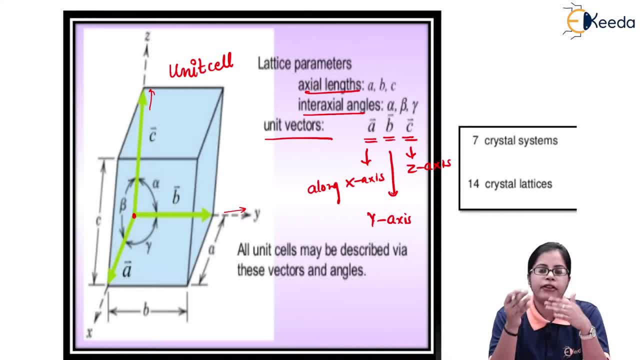 x and z. they have a certain angular separation, like alpha, beta and gamma. So this angles between the two axis is nothing but termed as interaxial angles. So if I have three axis, the angles between either two of them is going to be indicated as the interaxial angles. So alpha, beta, gamma is. 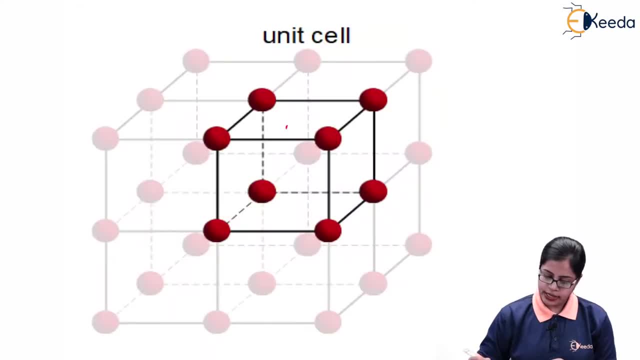 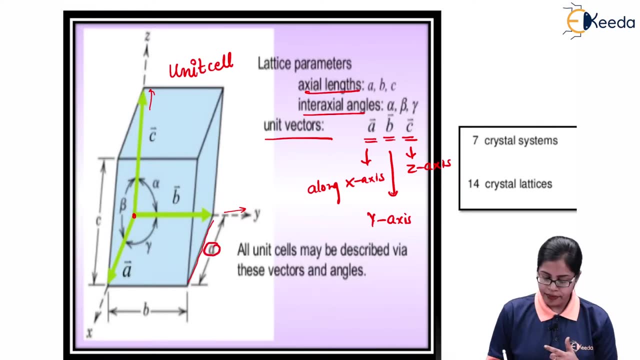 nothing but considered as the interaxial angle. Next, as you can see, the length of the unit cells, like this length is going to be considered as a. this length of the cubicle unit cell is going to be considered as b and this length of the cubicle unit cell is going. 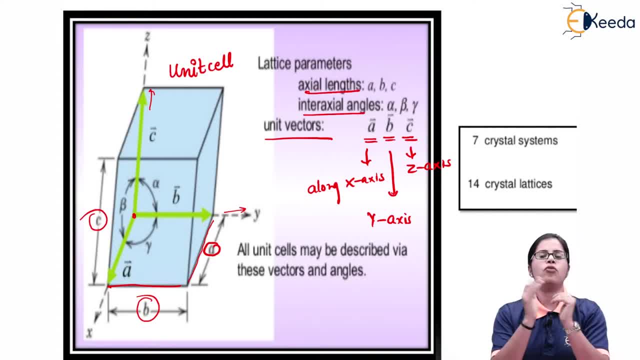 to be considered as c. So overall, if I look at the whole unit cell, I have to give three axial lengths, that is, a, b, c, three interaxial angles- alpha, beta and gamma- and three unit vectors, that is a vector, B vector and C vector. Now this is the lattice parameters, or we can say these are the three. 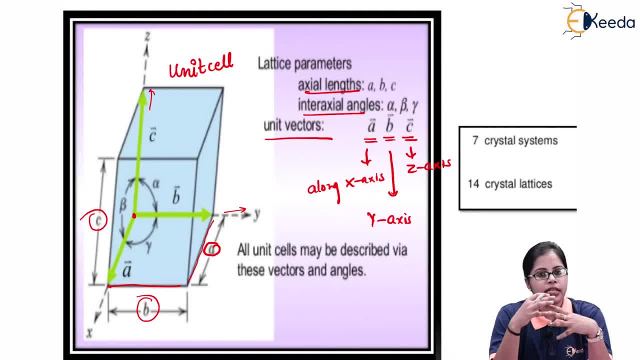 lattice parameters which we are going to make use of during the calculation of crystal structure. But when I make use of this unit, cells stacked together they are obviously going to lead to the formation of crystal structure. Now, depending upon the type of crystal structure I can have, 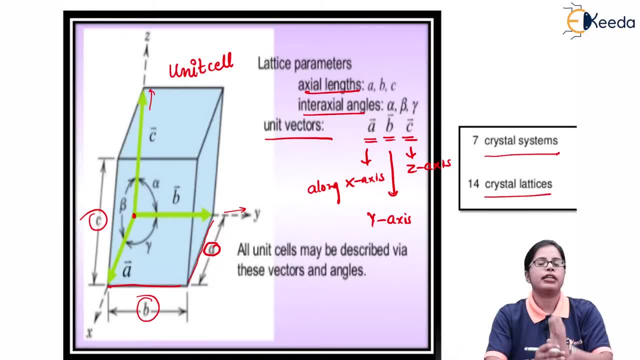 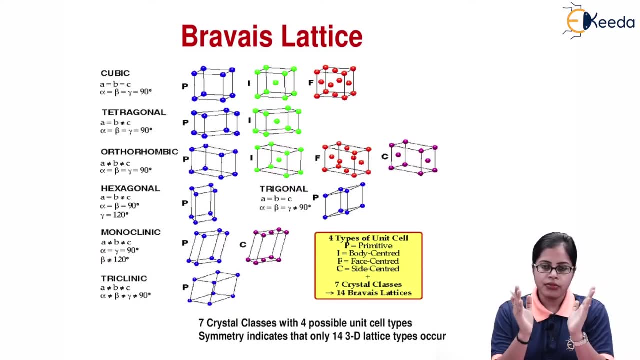 seven crystal systems and 14 crystal lattices. So this different systems are entirely dependent on the shape of the crystal structure. So what is this whole system called as? This whole seven crystal system is nothing but called as the Breville's lattice. Now, if you look at this, 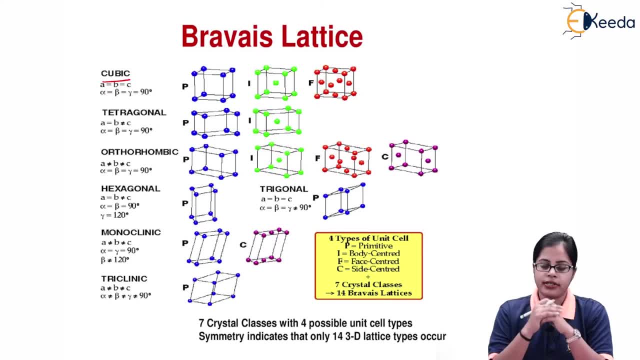 first one, it is the cubic unit cell, or the second one is the tetragonal. third one is the unit cell. fourth one is the unit cell and the fifth one is the unit cell. Now, if you look at this first one, it is the cubic unit cell, or the second one is the tetragonal. 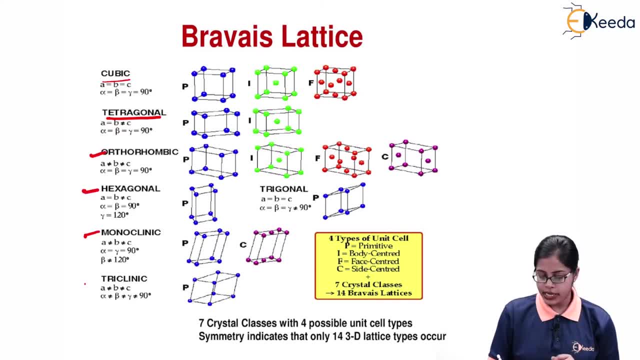 is orthorhombic, fourth, hexagon, monoclinic, triclinic and trigonal. so you have seven crystal system. but in between, as you can see, this unit cell is represented as primitive. this is represented as i, i means body centered. this unit cell is represented as f, that is face centered and overall. 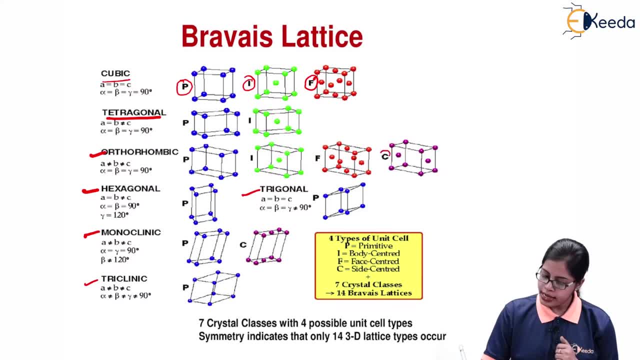 i again have the repetition of the same terms, but this c indicated has side centered. that means when you look at the whole system you have seven crystal system. that is cubic, tetragonal, etc. but when you look at the types of crystal latices you can have primitive type, you can have body. 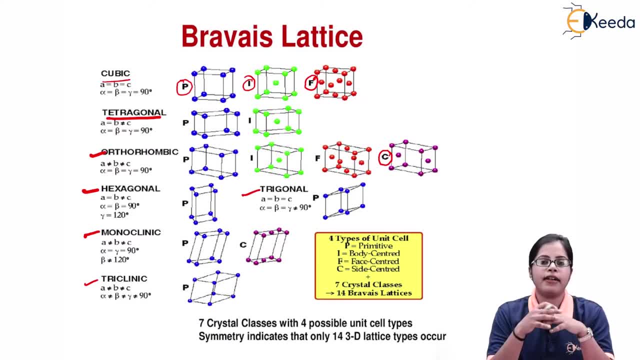 centered. we can have face centered or we can have side centered. so, using all these combinations, we have around 14 crystal latices. so these are considered to be the crystal systems, that is, and these are all considered to be the 14 crystal latices. so, depending upon the requirement that 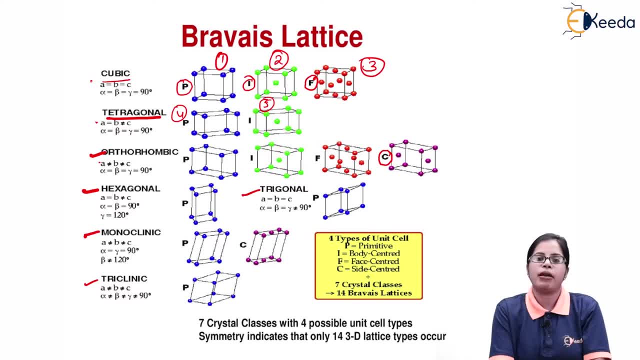 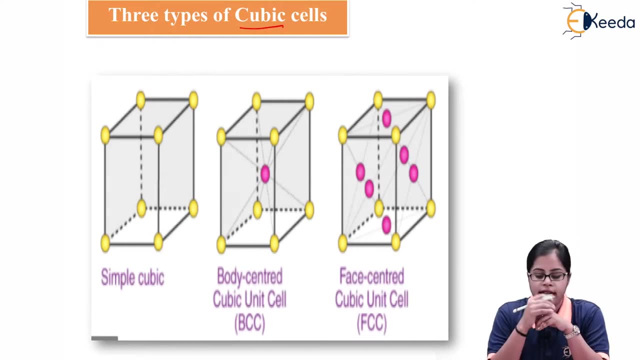 which type of crystal structure i require or which crystal system i am making use of. we are not going to classify the materials accordingly and we are going to make the crystals accordingly, but the most basic type of system which we make use of is cubic cells. that is the first one. as you can see, in the cubic cells all the actual lengths are equal, that is. 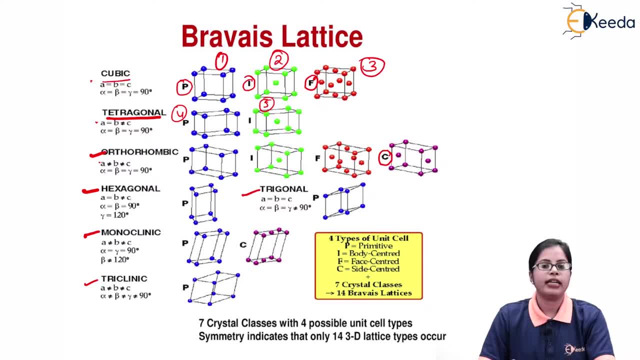 a is equal to b is equal to c and if you look at the inter-axial angles, that is, alpha, beta and gamma, they all are having a separation of 90 degree. that means the two axes, x, y, z or any of the two axis, are separated from each other at an. 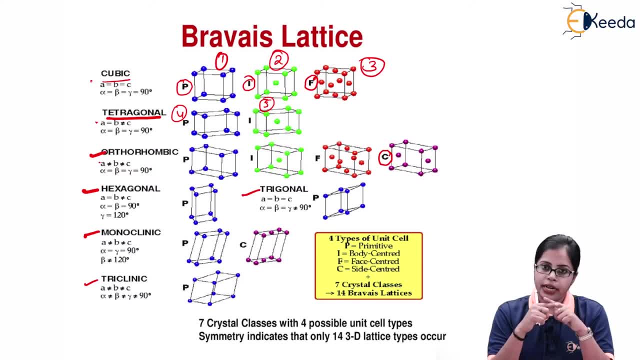 actual wavelength of the crystal system, so this one can be 12也可以 be defined as of 90 degree. so if they are separated at an angle of 90 degree, I can have the interaction angle value to be 90 degree for each of the cases. so for cubic unit. 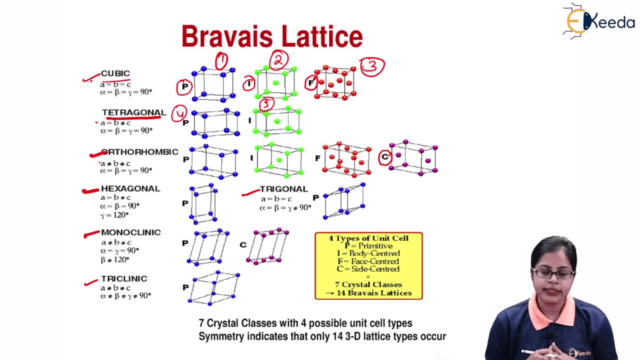 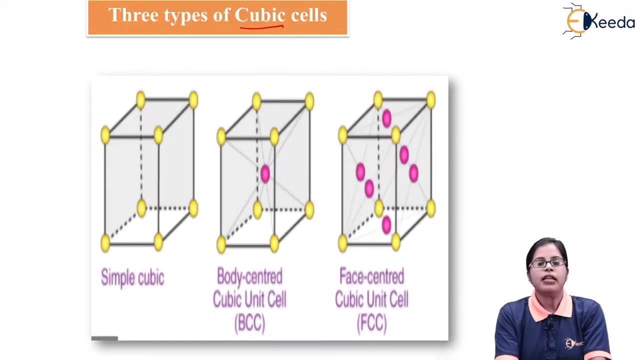 cell. we have equal interactual angles and equal axial length and, if you can see in this cubic unit, cell is of three types. that is primitive, and sometimes this primitive is also called as simple cubic cell. i is indicating the body centered and F is indicating the face centered. so let's talk about the three. 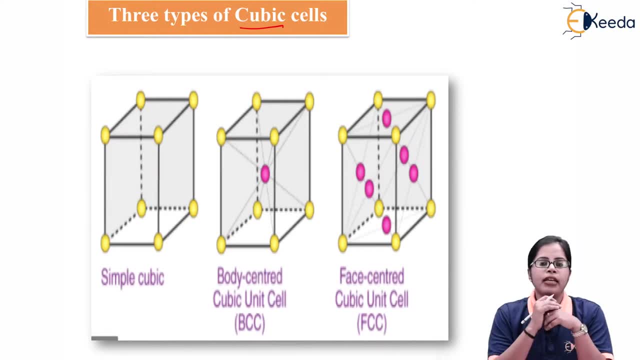 types of cubic unit cells. now, as I said, in the cubic unit cell we have equal axial length, that is, a is equal to B, is equal to C and the interactual angles are all equal to 90 degree. that means, again, the interactual angles are equal. 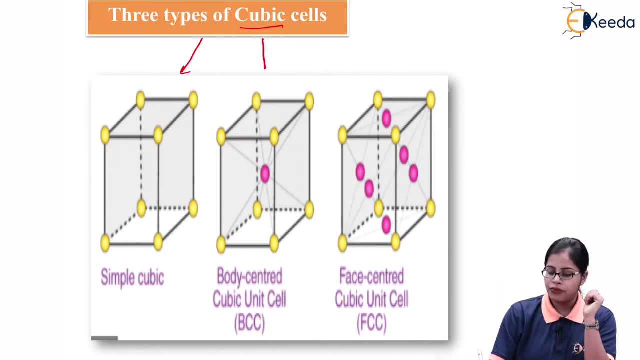 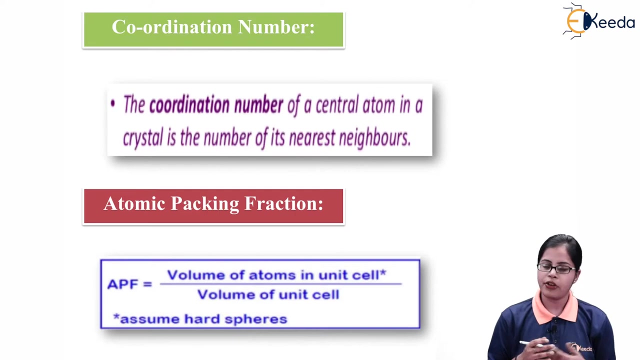 to each other and once you look at the classic of cubic unit cell, they are classified as primitive means simple cubic. I, that is body centered, and F is considered to be face centered. so cubic cells are going to have three types: primitive, that is simple cubic cell. I, that is body. 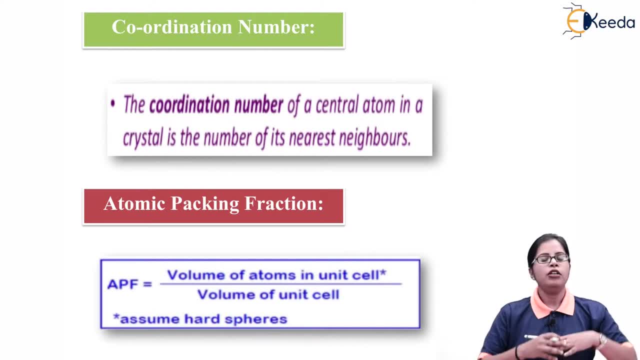 centered F, that is, face centered. now, before going in the description of that, what do you mean by simple cubic cell, or what do you mean by body centered, or what do you mean by face centered? we are going to talk about the two main parameters which we are going to make use of during the calculations of 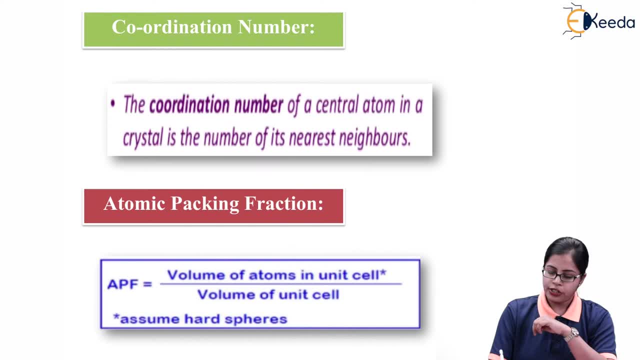 different cubic cells. the one is coordination number. now, when you say coordination number, in this case we are trying to calculate the number of nearest neighbor to a central atom. so if I consider a central atom and if I calculate the number of nearest neighbor around the central atom, 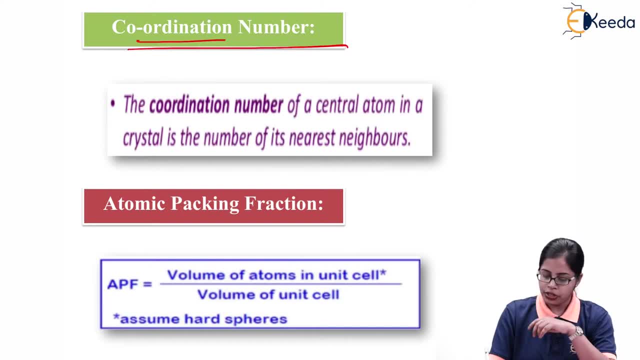 that number is considered to be the coordination number. secondly, we are even going to talk about atomic packing fraction. atomic packing fraction is nothing but considered to be the volume of atoms in a unit cell divided by the whole volume of unit cell. so we are going to make use of two important parameters. 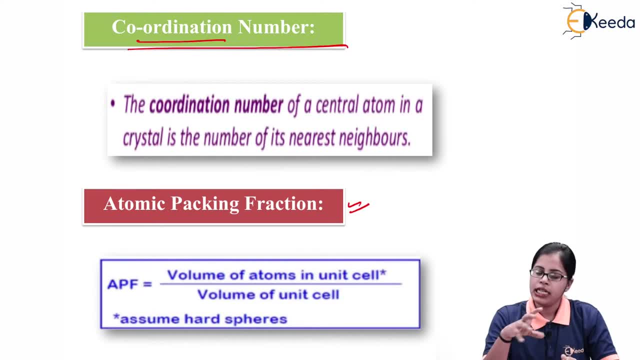 that is coordination number and the atomic packing fraction. so if I calculate the number of nearest neighbor to a central atom, that number is indicating the coordination number. secondly, when you're talking about atomic packing fraction, this gives you the formula, obviously, but when you talk about atomic 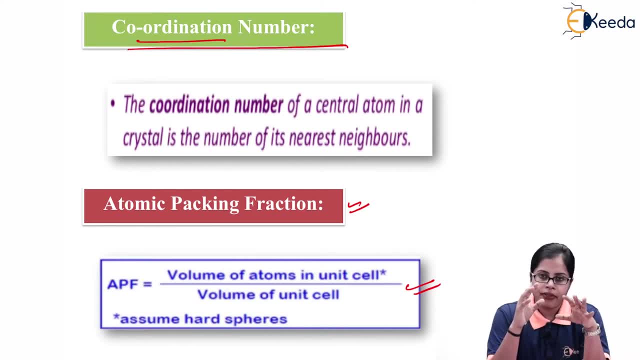 packing fraction? what do you mean by it? is that how much part of the unit cell is completely packed with atom? or how much fraction is roughness to avoid? well, if you're using a throw, a logic, formula, a, the raw, that's all known about breaking bottom and 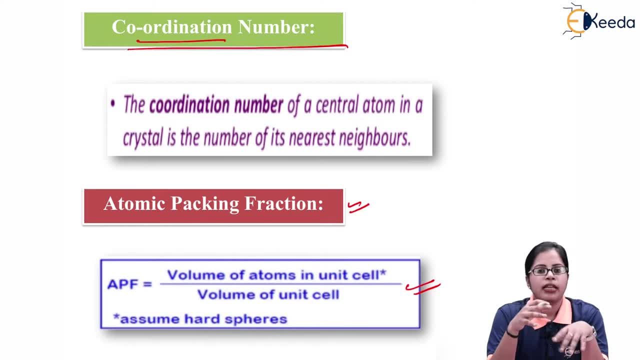 of unit cell is packed with atom. that concept is called as atomic packing fraction. So if you want to calculate atomic packing fraction, we need to know what is the volume of atoms in unit cell and what is the volume of units in. So we have to remember one thing very well, that when we talk, 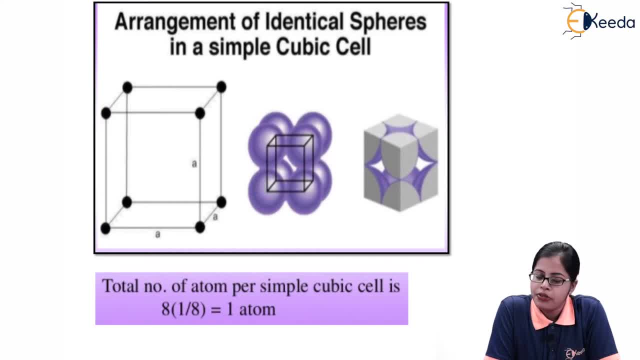 about atoms. atoms are considered to be spherical in shape, So when I say volume of atom it should be the volume of sphere. Secondly, when I say volume of unit cell, we mean to say unit cell is of a cubic shape. So as we have considered cubic unit cell, so volume of a cubic unit cell is nothing. 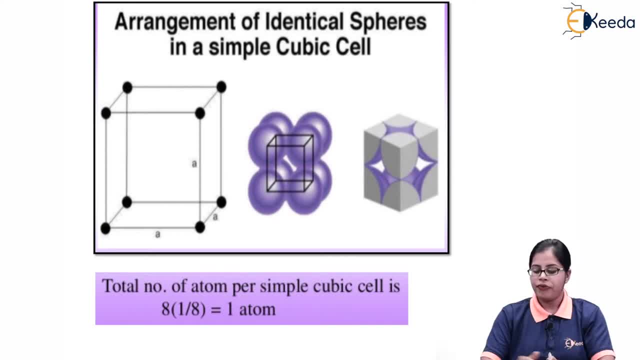 but the cube of the length of the cube. So now, when we are starting with the calculations of different type of unit cells, that is, different type of cubic unit cells, in that case we have to know what is the volume of atoms in unit cell. So when I say volume of, 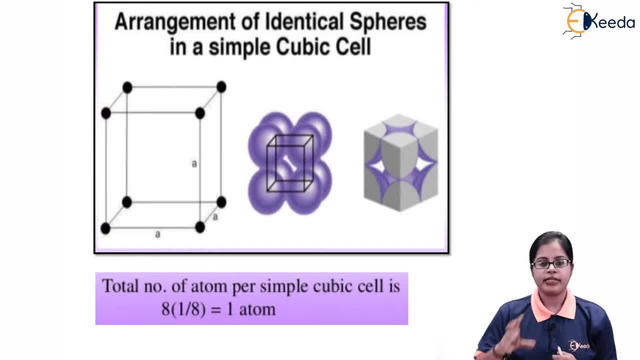 atoms in this case. first, we are starting with the simple cubic cell, that is, the primitive unit cell. Now, when you say primitive or simple cubic cell, in this case, as they are representing cube, the length of each side of the cube is going to be equal as the for cubic unit cell, the actual lengths are: 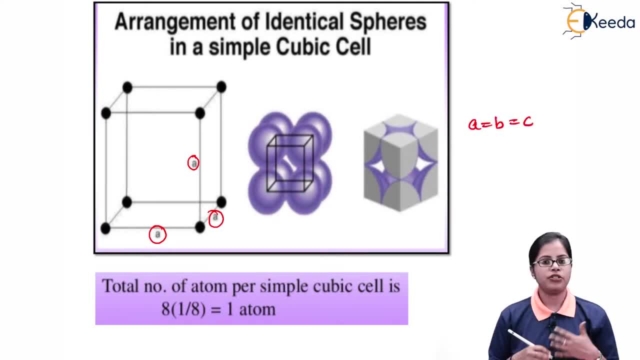 equal. So we can have: a is equal to b is equal to c, So I can just represent all the length to be same. that is the length of the cube. So we can have: a is equal to b is equal to c. So I can just. 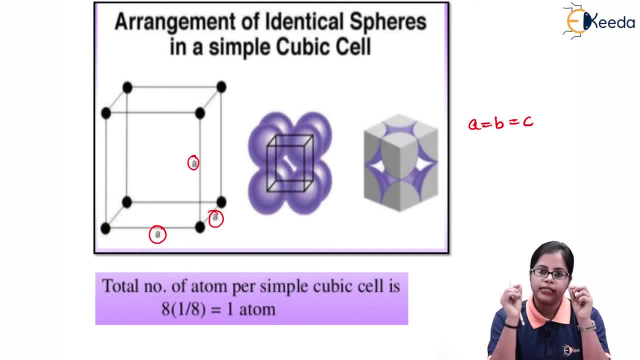 say the volume plot of the cube, well as a. The second thing: as you can see, the atoms or the lattice points are arranged at the corners of the cell. that means if I consider unit cell which is of cubicle shape, I will have eight corners. So all the lattice points, or all the bases are going to be attached to. 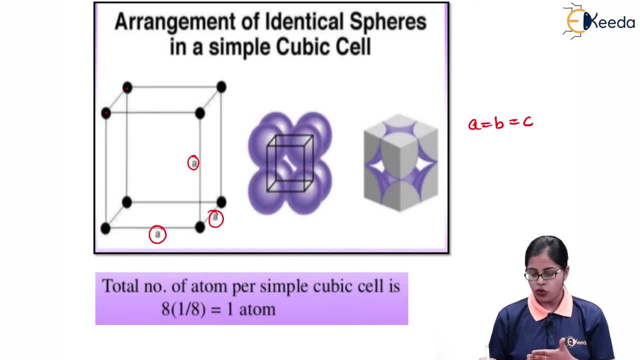 the 8 corners of the simple QUBIC cell. next is when we talk about the total number of atomsciores present wage a simple cubic cell Summit. number of atoms is the quantity of this attached single cell and the total number of atoms which are present per simple cubic cell is equal to at a single cubic heel. this'. 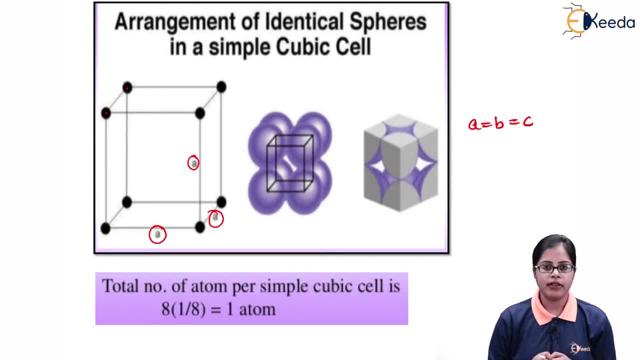 the total number of atoms. this, i mean, is equal to every thing outside. so the total number of atoms are equal to two times the number of atoms in every single house per cubic cubic cell which are present per simple cubic cell. what happens over here is like we have. 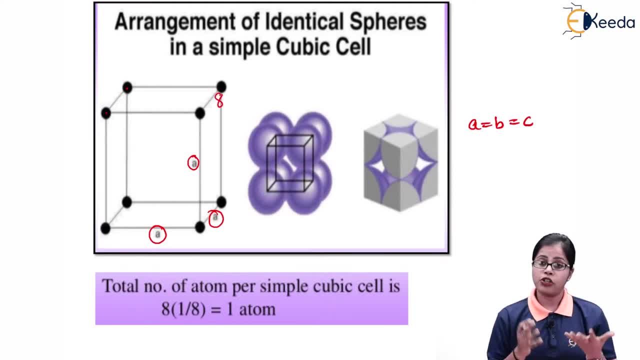 total eight atoms, but not for a cubic unit cell. we are talking about the whole crystal structure. but if we have eight atoms, but when we talk about the separation or division of atoms in terms of unit cell, so the eight atoms I divided 1, 8th time for the unit cell. so if I consider 1, 8th of 8 atoms, that is 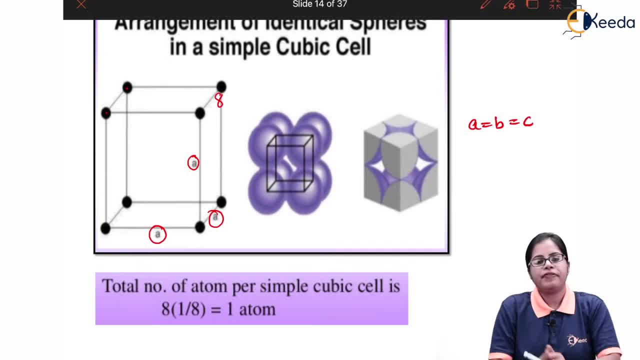 going to give me one unit cell. so when we are talking about the three types of cubic unit cell, the one we are talking about is a simple cubic cell. in this case, simple cubic cell is also termed to be primitive, and when we talk about primitive, what we mean by primitive unit cell is that all the layers 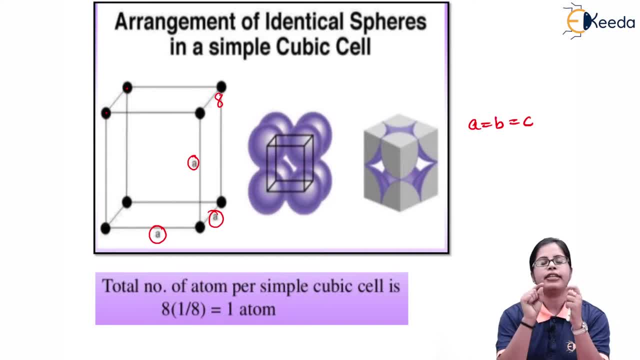 lattice points are attached to its corner. so if the lattice points are attached to only the corners of the unit cell, that type of unit cell is considered to be the primitive unit cell or the simple unit cell. and secondly, as it is a cubic unit cell, the axial length are going to be equal to each other. so 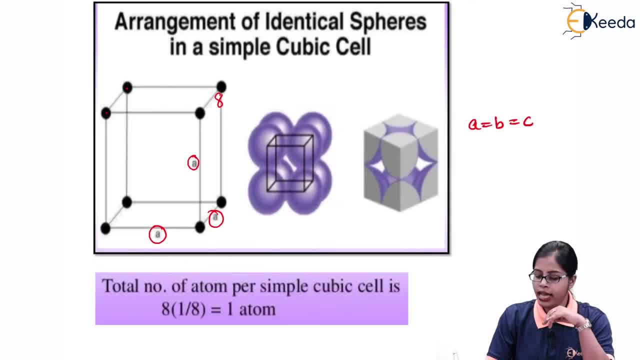 that is why we can say that A is equal to B is equal to C and that is why I've termed all the length to be as A. secondly, when we talk about the three types of unit cell, we are talking about the three types of unit cell. we are talking about the three types of unit cell. we are talking about the. 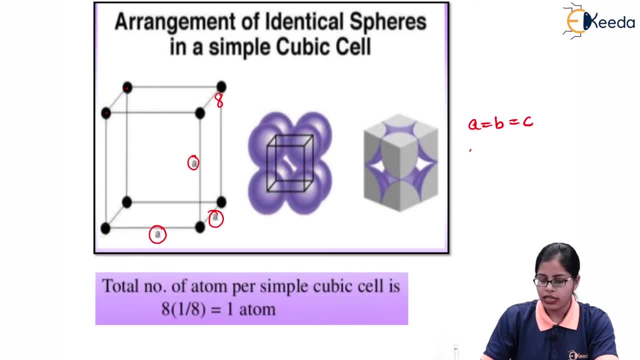 simple cubic cell in the 3d array. so in 3d array, if we consider a simple cubic cell, in that case each atom of the unit cell is going to be shared or linked with eight unit cells or the eight neighboring unit cells. so in 3d figure, 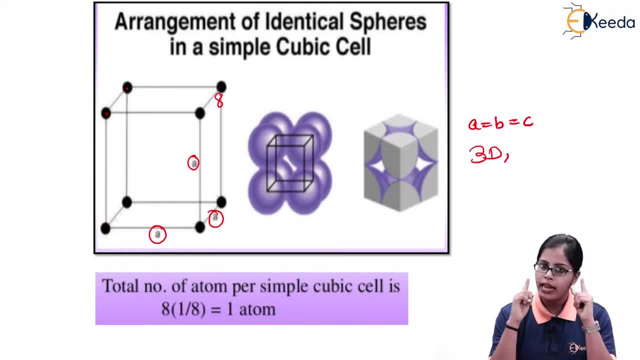 we can say that each atom is going to linked with the eight neighboring unit cell. that means each atom, one eighth part of each atom, is going to link to the one unit cell. that means when we talk about the number of atoms which are linked to one single unit cell is going to be represented as like. if I consider a 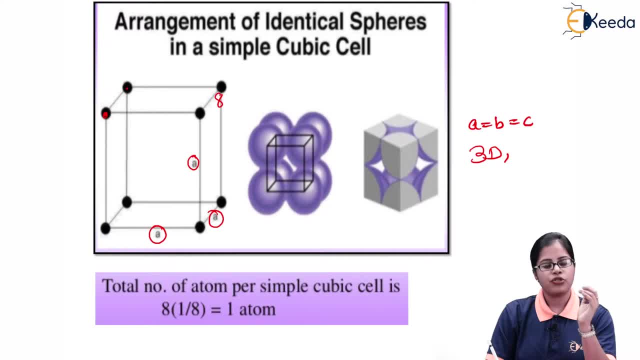 single atom over here. this single atom is going to link to the eight neighboring unit cells. so for one unit cell, the at them one eight content is only going to occur. so if I say one atom is going to get link to the 8th unit cell, so that means one atom is going to consider for. 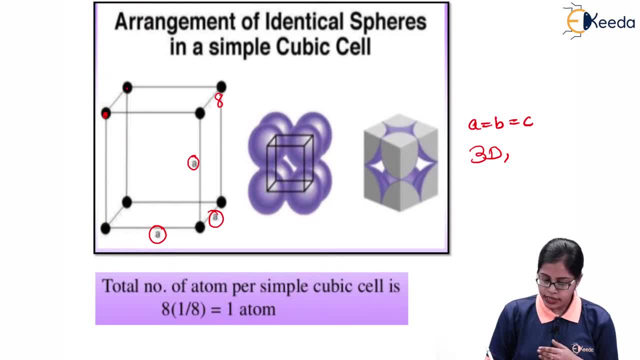 the 1- 8th time. so, when you take the number of atoms which are present per unit cell, we are going to take it as has. one single atom is shared by 8 unit cells and we are going to select one single atom as 7 times and into the other cell. 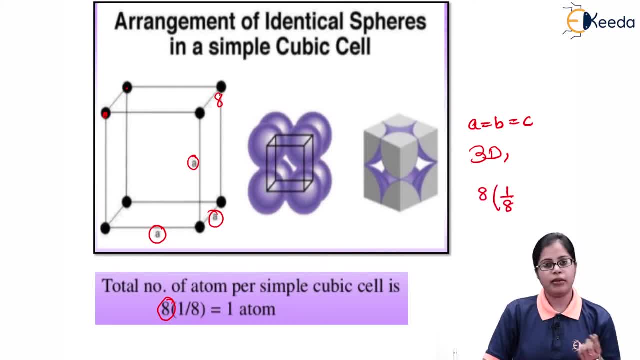 so 1, 8th of its content is going to be available for each unit cell. so the number of atoms which are available per unit cell is going to be the 8. into 1 8th of the 8 unit cells is equal to 1 atom. 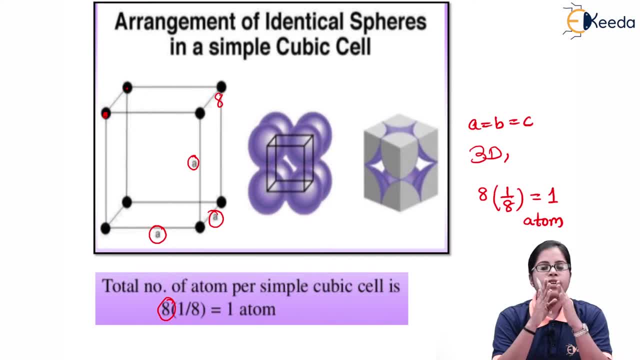 so one single atom is getting contributed or linked to 8 unit cells and that means if we divide the content of one single atom it is going to get divided one eighth the time. so 1 8th of 8 is going to give me one atom for single unit cell of simple unit cell or a simple 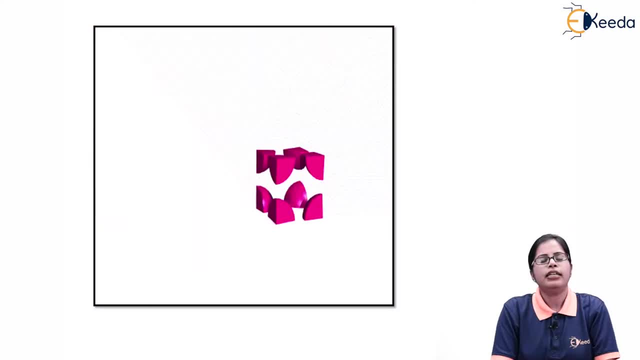 primitive cell. so if you want to know that, how many number of atoms are present in a simple cubic unit cell, that is the one eighth of the whole contribution. that is one atom present in a simple cubic unit cell. that is one eighth of the whole contribution present per unit simple cubic cell. Next is this is how, if I make use of a simple unit cell, 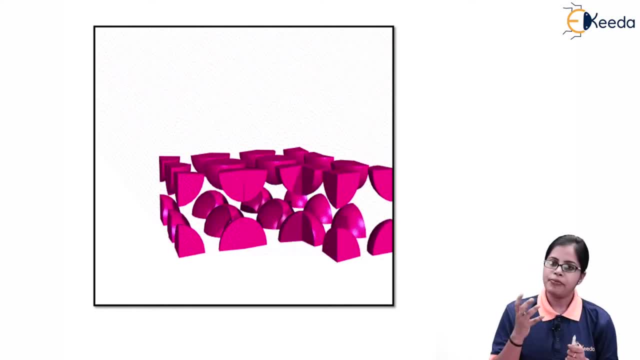 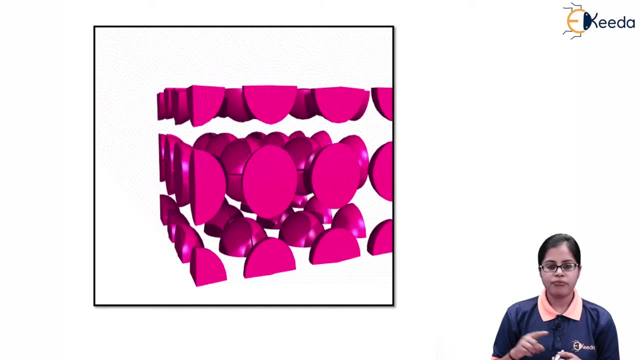 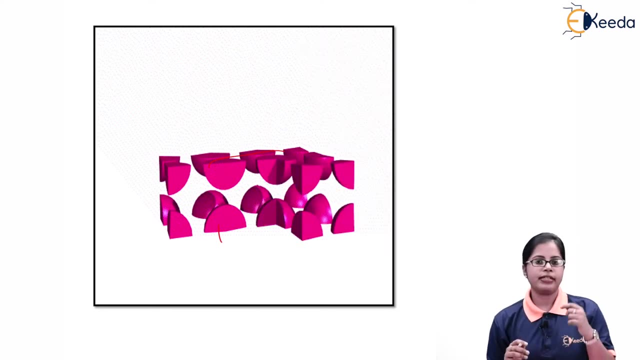 and if we keep on attaching or stacking simple cubic unit cells together, this is how the 3d figure of the crystal is going to form. So this 1: 1 block, or this 1: 1 basic building block, is considered to be the simple cubic unit cell consisting of one atom per unit cell. 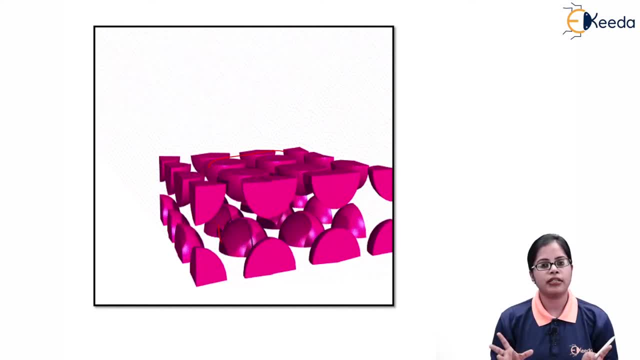 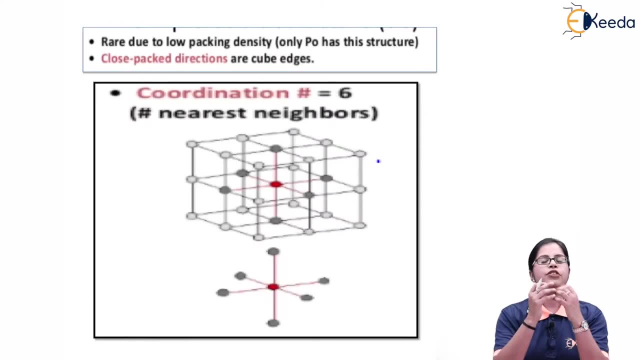 and if I keep on stacking all these unit cells together, we are going to get the simple cubic crystal structure. Next is when we talk about this simple cubic unit cell. as I said, I have only one atom per unit cell, So that means they have low packing fraction because they have only 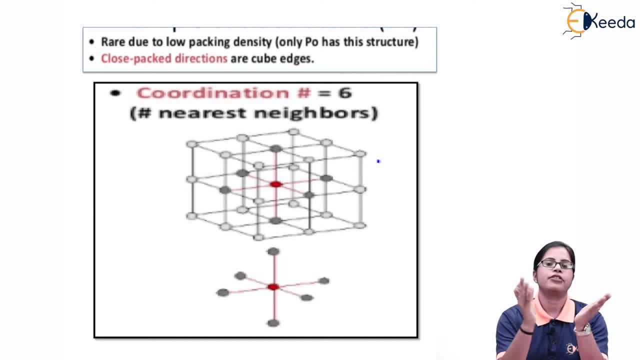 one atom present in one unit cell. So if I keep on taking the crystal structure, In that case the unit cells are stacked together, giving me a crystal structure. So if I have only one atom for one particular unit cell, so the packing fraction is very less means the number. 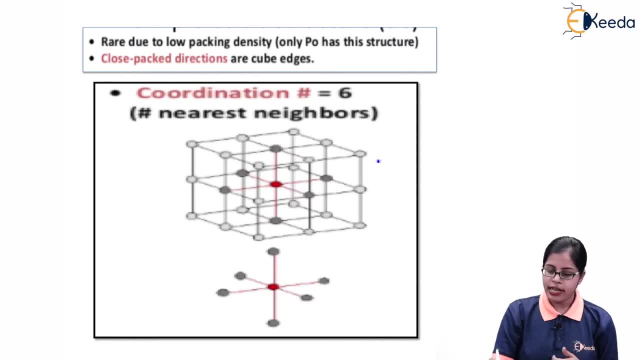 of atom available for a unit cell is very less So, as they have low packing density, they are very rare and the only example which we have is polybidynum for simple cubic unit cell, because they have low packing density, that is, they have only the presence of 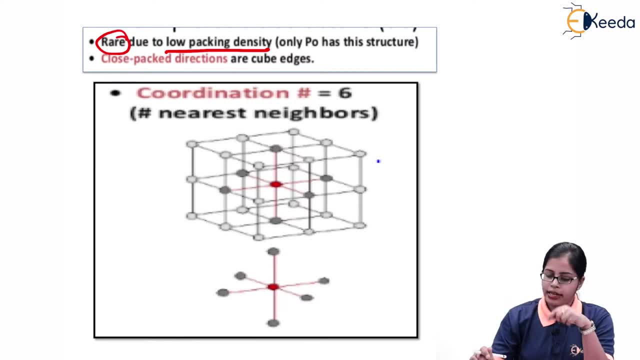 one single unit cell. So if I keep on stacking all these units together, they are very rare. They have one single atom per unit cell and they have a closed packed structure and they have cubic edges. now, when we talk about the coordination number, I have already talked about the 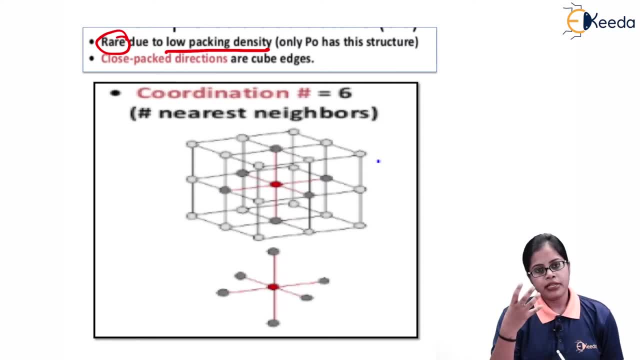 coordination number is that? coordination number is the number of nearest neighbor attached to a central atom is going to be called as coordination number. Now this red one is behaving has a central atom and, as you can see in the diagram, there are 1,, 2,, 3,, 4,, 5 and 6.. That is we can say we have 6 nearest neighbor to the central atom. 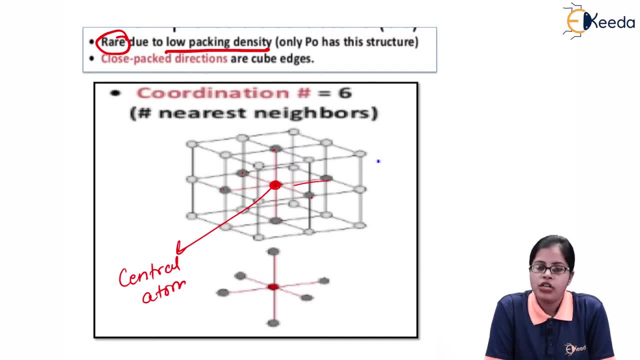 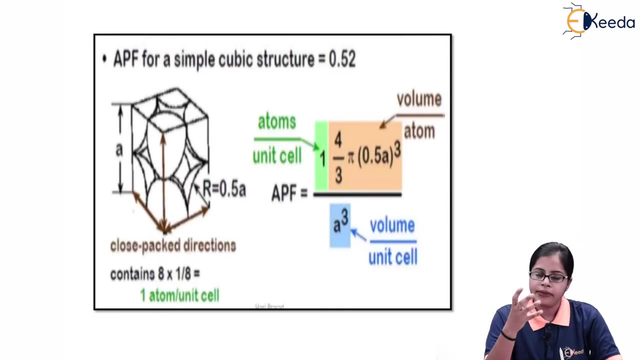 So if I get to know how many number of nearest neighbor I have to a central atom, in that case we can say that the nearest neighbor to the central atom is 6. So the coordination number is considered to be 6.. Next is: if we want to calculate that, how much is the atomic packing? 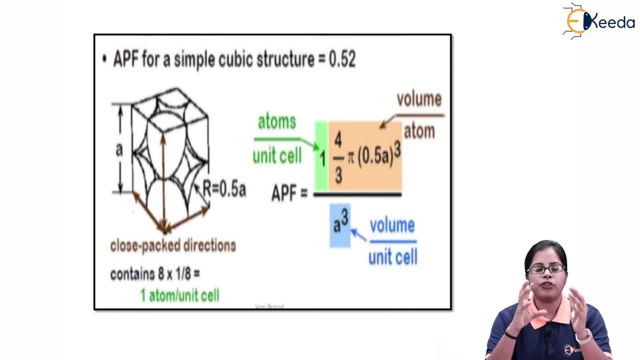 fraction of cubic structure, that how many part of the unit cell is packed with the atom. In that case we need to make use of the formula that the volume of atoms in unit cell divided by the volume of unit cell. So if we consider that formula, that means atomic packing fraction is nothing but. 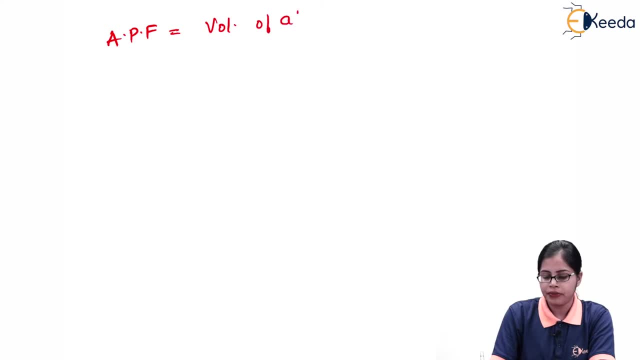 the volume of atoms in unit cell divided by the volume of unit cell. And, as I said, atoms are considered to be spherical in shape and unit cell is of cubic shape. So if I want to get to know what is the volume of atom in unit cell, we need to first of all know that how many number of atoms 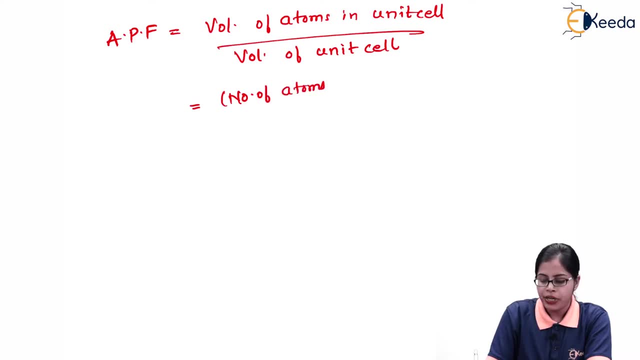 are present per unit cell into the volume of atom, The whole divided by the volume of unit cell. Now, as we are aware, so when we are calculating the atomic packing fraction, we said that it is volume of atoms in unit cell divided by the volume of unit cell. So if we were to 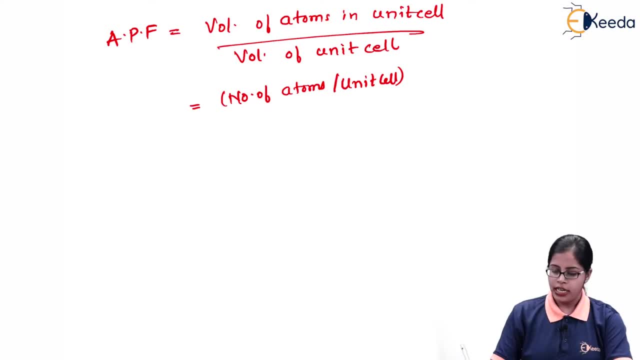 calculate what is volume of atom in unit cell. we need to know that. what is the number of atom present per unit cell? volume of atoms, or you can say volume of each atom and the whole divided by volume of unit cell. now this is simple cubic unit cell, or you can say the primitive unit cell. 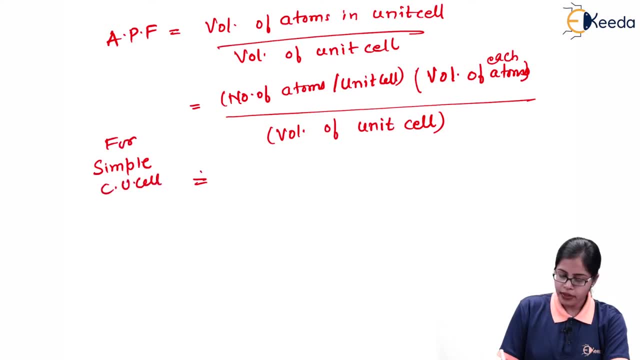 so for simple cubic unit cell we can have or we are aware that there are one number of atom per unit cell. as we are aware, the number of atoms which is present per unit cell is one. volume of each atom is going to be considered as 4 by 3 pi r cube, as atom is represented as a. 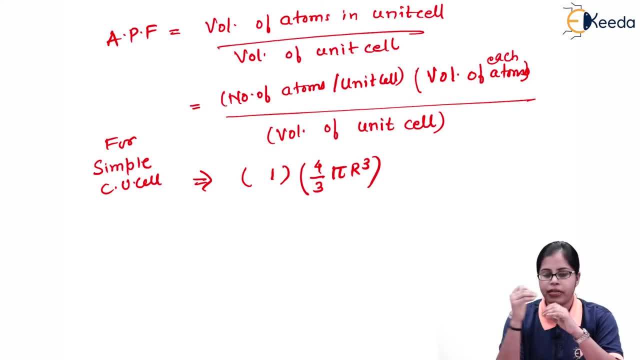 spherical shape. so the volume of the sphere is 4 by 3 pi r cube and r is considered as a spherical shape. so the volume of the sphere is 4 by 3 pi r cube and r is considered to be the radius of each atom. secondly, when you consider the volume of unit cell, in that 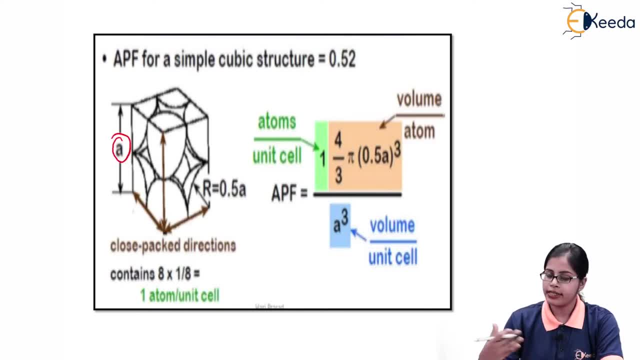 case, the length of the unit cell is taken to be a. as it is a cubic unit cell, the volume is going to be the a cube. now, when you look at the value of radius of the atom, in this particular simple cubic unit cell, radius is taken to be 0.5 a. that is half of. 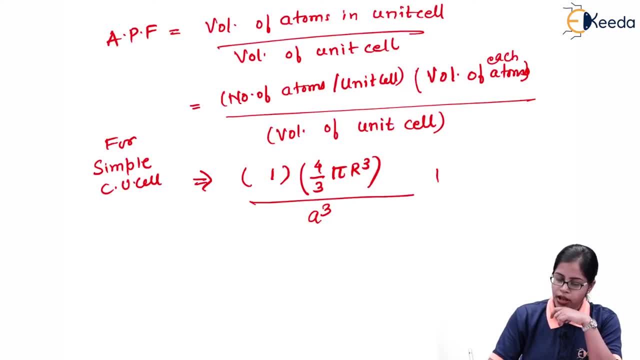 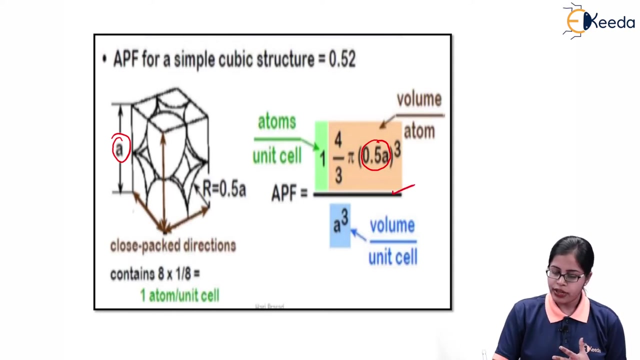 the length of the unit cell. so instead of r we can make use of 0.5 a value, as r is indicating the radius of atom and 0.5 times of a is representing the actual length of the unit cell. so once we calculate the whole value by substituting everything, in this case we get the atomic 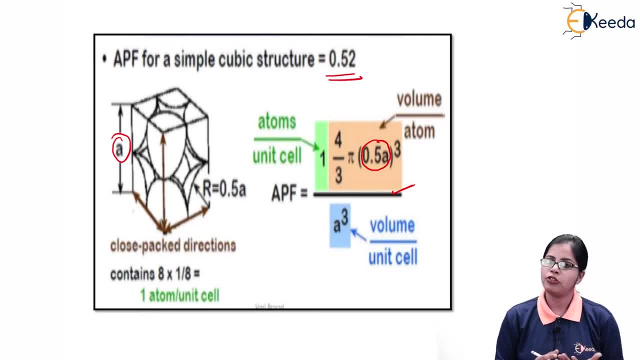 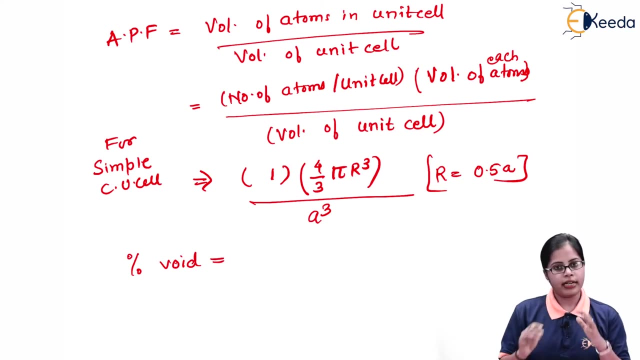 packing fraction of simple cubic structures to be around 0.5- 2. so this is giving me that how much part of the simple cubic unit cell is filled with atom and if we want to calculate that, how much percent void is present in that simple cubic unit, sin once if I get the value of atomic. 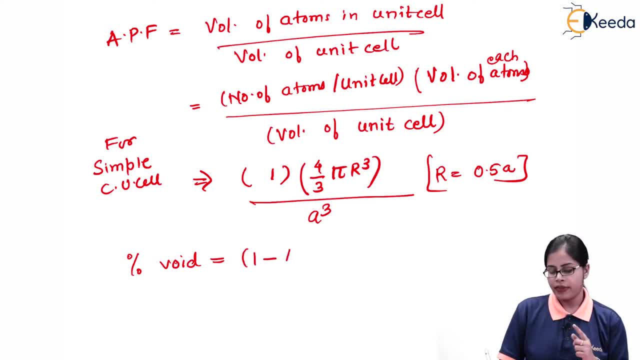 packing fraction. just subtract the atomic packing fraction by 1 times 100 will give me the value of the percentage of void which is present in the unit cell. What do I mean by void? Void means empty spaces. So if I say the atomic packing fraction, 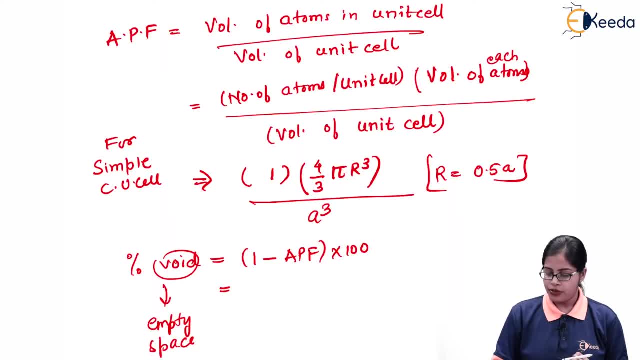 of simple cubic structure is around 0.52.. So if I calculate the percentage of void present in the simple cubic unit cell, it is going to be around 0.48 times 100.. It is going to give us 48%. So 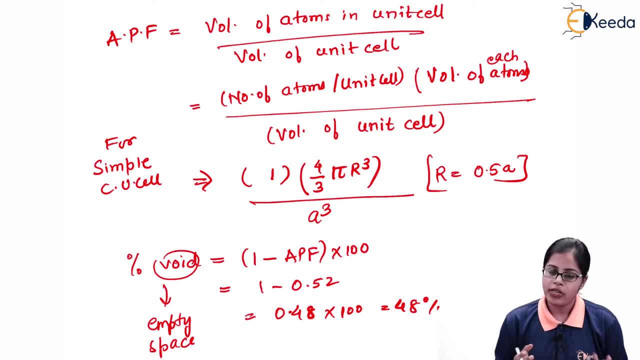 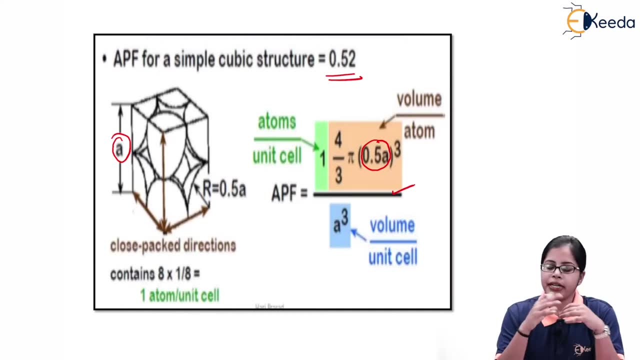 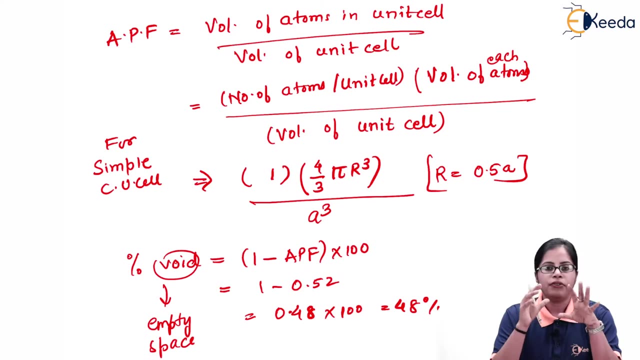 48% of the simple cubic cell is empty, or you can say it is void, and 52% of the simple cubic unit cell is packed. So this is how you calculate the atomic packing fraction, coordination number and the percentage void of the simple cubic unit cell. 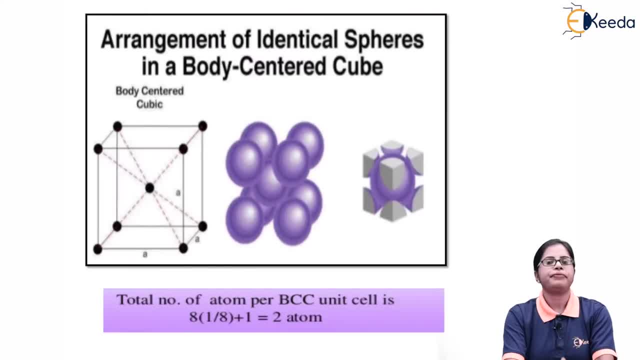 So this is the first type of cubic unit cell, that is, simple cubic unit cell. Next is the second common type of simple cubic unit cell is considered to be the body centered In body centered cubic unit cell. we have the placement of the lattice points at all the eight corners of the cubic. 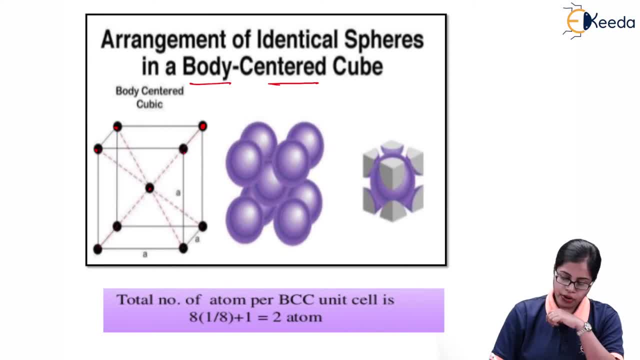 unit cell. plus we have one more lattice point attached at the center of the cubic unit cell. So this is the placement of the lattice points at all the eight corners of the whole body of the cubic unit cell. That means we have eight lattice points attached. 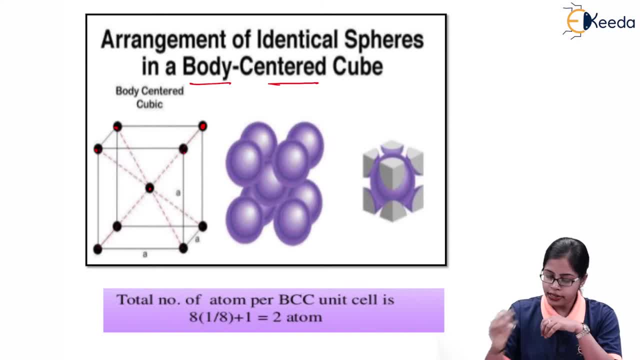 at the eight corners of the whole cubic unit cell and one lattice point attached at the body or the center of the body. So if you look at the whole number of atoms present in the body centered in this case, we can calculate in two manners. 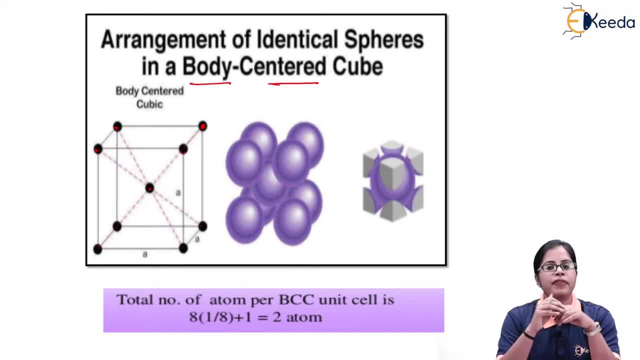 The same thing, like the way we talked about the simple cubic unit cell, that one atom at the corners are linked to the eight unit cells. So eight unit cells are going to be linked to one single atom and if we talk about, each atom is going to have one eighth part of its 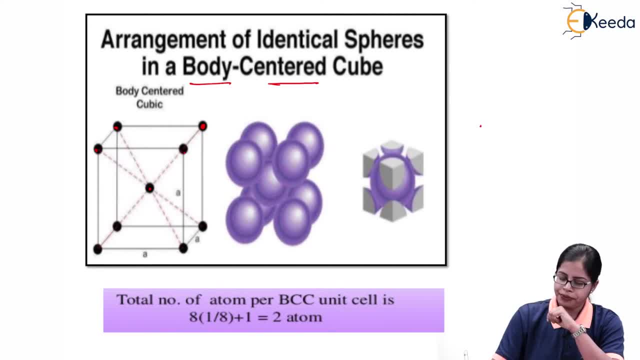 content in our single unit cell. So if I have one single atom getting linked to the eight unit cell And for each unit cell we have the availability of the one eighth of its content, Then that is going to give me the one atom from the corners of the lattice points and as we are, 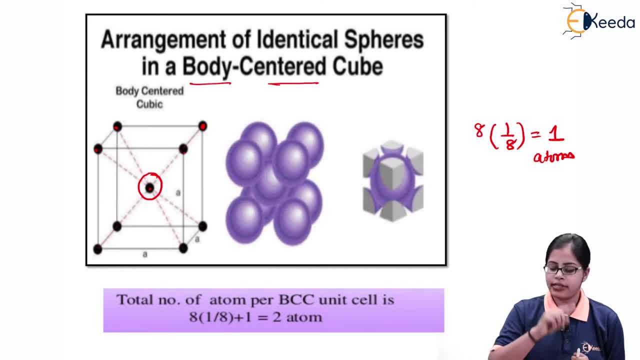 already aware that there is a one more atom which is present at the center. So there is already one atom present in the unit cell at the center. So this one atom is contributed by the corner and this one atom is already present at the 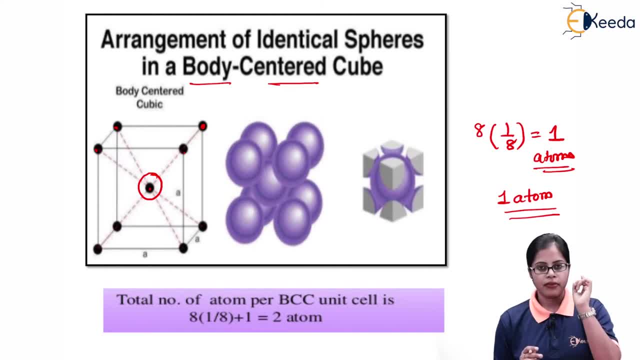 center. So the total number of atoms which is present in the body centered cubic unit cell is 2. One which is given by the corners, that is, one atom is contributed by the corners and one atom which is already present at the center of the cube. So overall, if you look at the number of 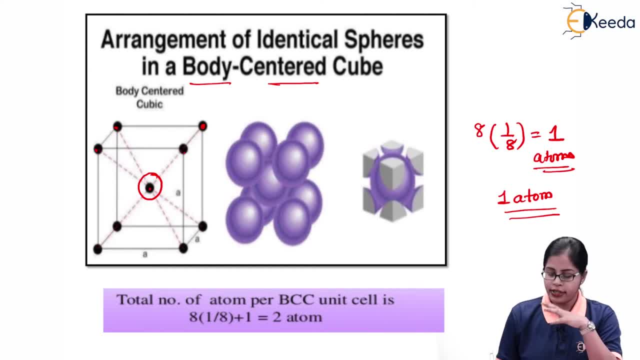 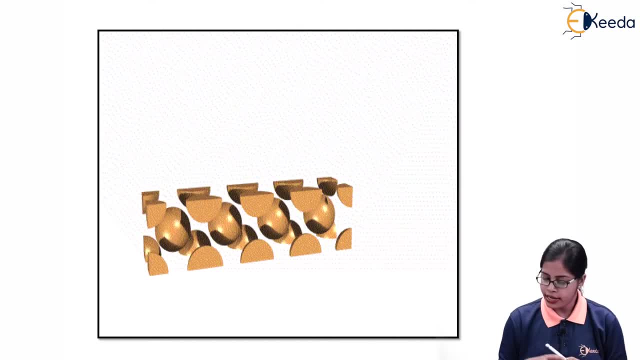 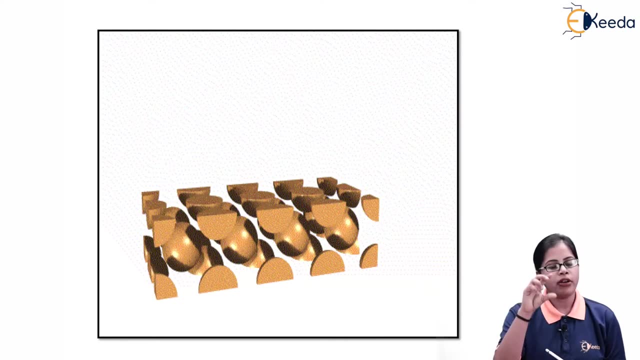 atoms which are present per body centered unit cell it is going to be two atoms. Next is: this is how the body centered unit cell looks like. So this whole one, one stack or one one part, is indicating the body centered cubic unit cell. and if I keep on stacking this body centered unit 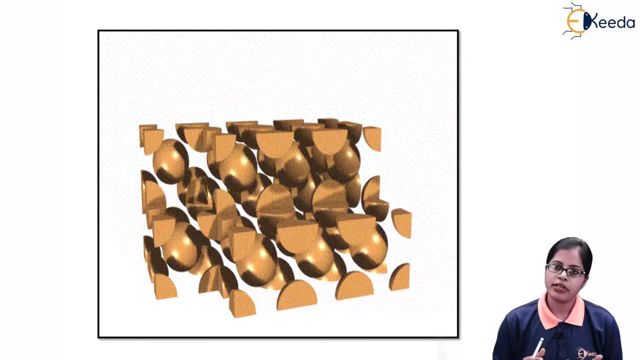 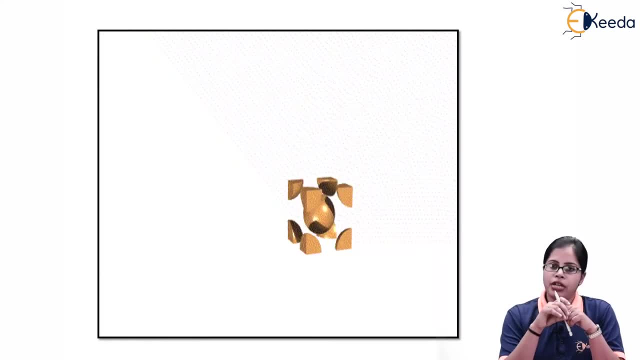 cells together, we are going to get a crystal structure having a body centered lattice. So if I keep on stacking this body centered unit cells together, we are going to get a crystal. If you want to make a body centered lattice, a single unit cell should have two atoms, that is. 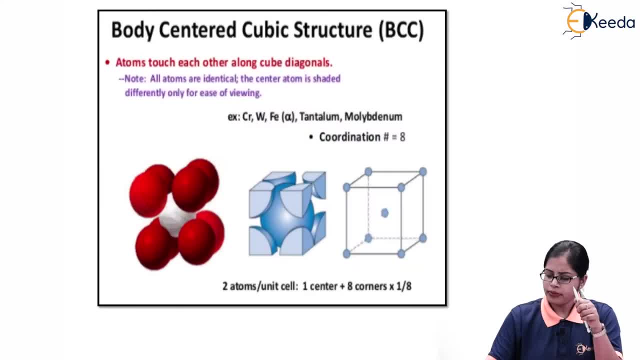 what is going to lead to the formation of body centered crystal, and one important part in this is that when we talk about the body centered, there is always a presence of atom at the center of the body. Next is, as you can see, that there is one more, like at the eight corners. we have eight. 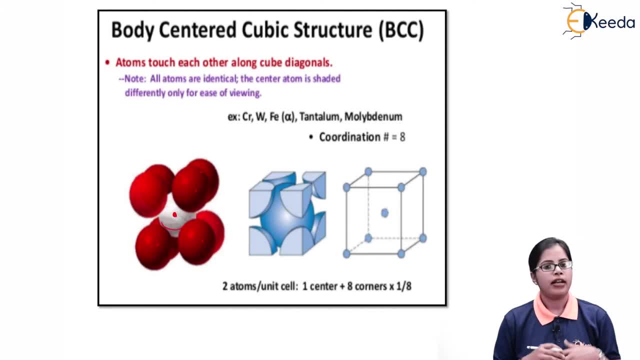 lattice points and we have one atom which is present At the center. so we can say that the atoms touch each other along the cube of the diagonal. or we can say, in body centered atoms touch each other along the diagonals of the cube, like these are the two. 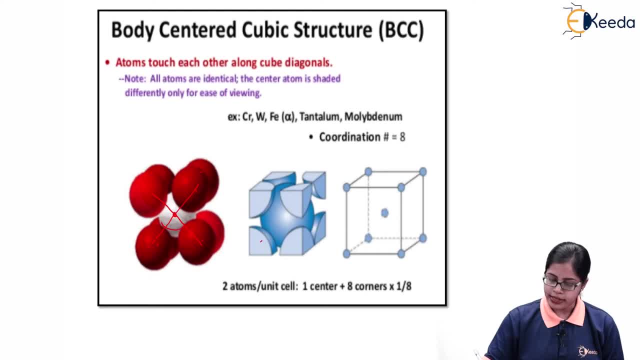 diagonals you can draw, as you can even draw this diagram like this: this is one diagonal of the cube. so in BCC, or in the body centered cubic structure, we can say the atoms are linked with each other or can be touching with each other with the help of the cube diagonals. and second thing, has all atoms. 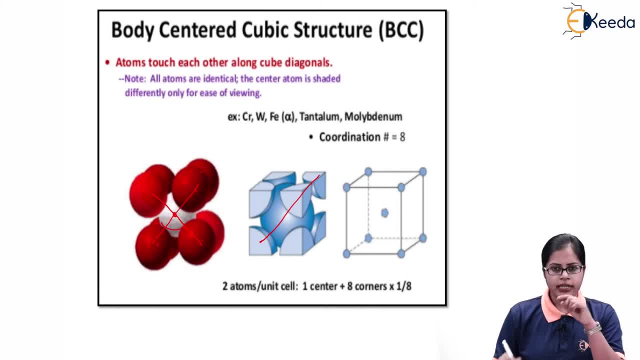 are identical and at the corners and the center one is also identical. that means all the atoms which are present in the unit cell are entirely identical, but just for differentiating that we have one more atom present at the body centered. that is why we have the made use of white shape. 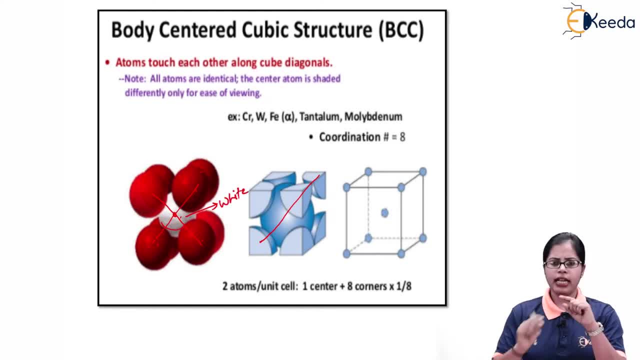 For the body centered one and the ones which are present at the corners, they are shown by the red shape. so it doesn't mean that when you change the shade of the colors over here it means that all the atoms are going to be same, just for the angle of viewing, that which atom is present where we are. 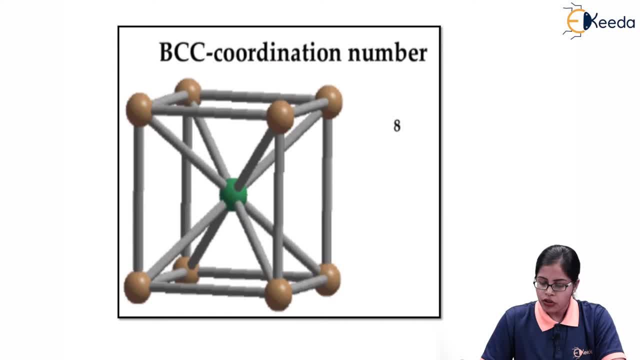 just making use of different shades over here now. secondly, when you talk about the coordination number, that is, number of nearest neighbor To the central atom is going to give me the coordination number. so if I look at the central atom, this green one indicates the central atom and, as we can see, there are eight nearest neighbors to the central atom. so 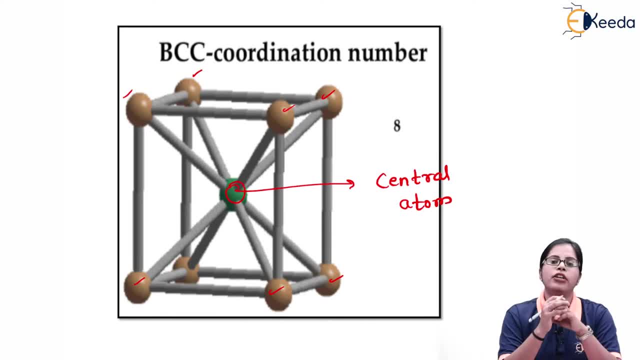 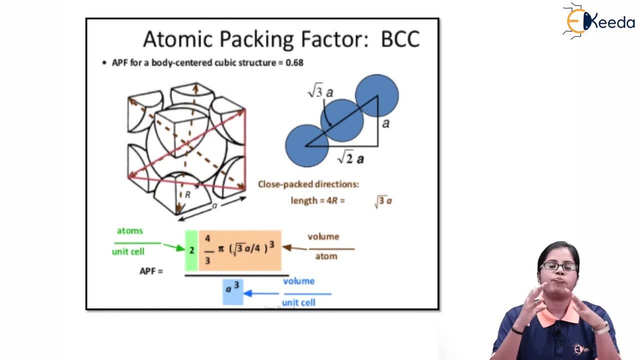 the coordination number of the central atom, or you can say the coordination of the body centered cubic unit cell, is going to be eight. now if you want to calculate how much part of the body centered unit cell is packed and how much part is void, in that case we have to make use of again the 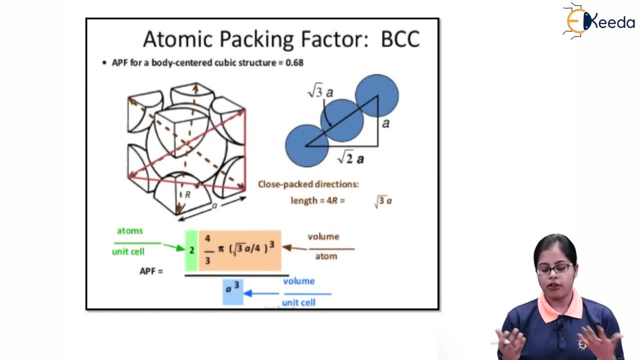 calculation of atomic packing fraction. and the atomic packing fraction is only been calculated in the terms of atoms per unit cell, into the volume of each atom divided by the volume of the unit cell. so if we talk about the volume of each atom, again atom is of spherical shape, so the volume is going to be. 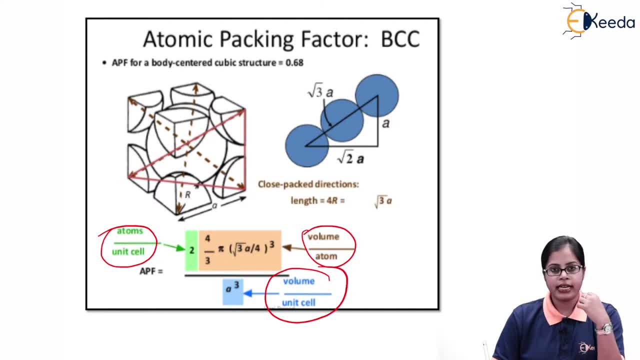 4 by 3 pi r cube. but in this case when we take the radius of the atoms, we get the radius of atom to be around root 3 a by 4, and a is obviously indicating the actual length. and if we look at the whole shape of the 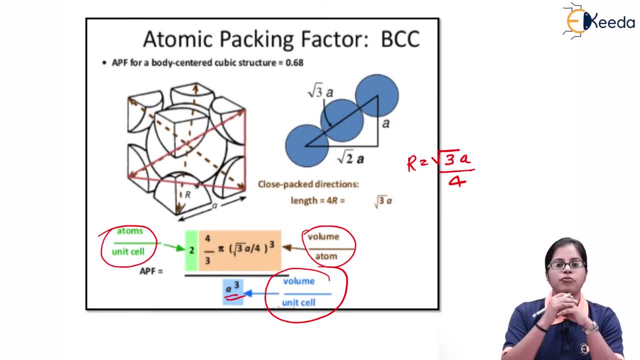 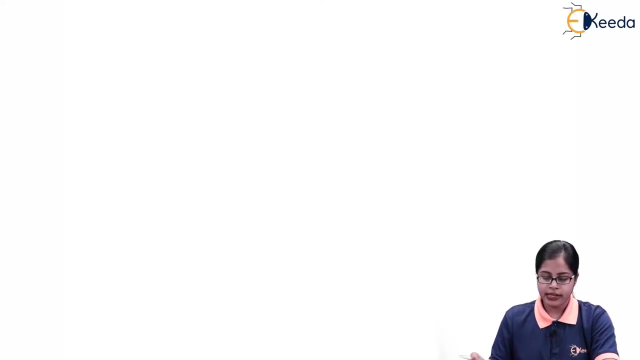 crystallitis cubical shape. so the volume of the unit cell is going to be a cube. and if you want to get to know what is the atoms per unit cell, we have already calculated For body centered. the number of atoms which are present per unit cell is 2. so this term multiplication together is going to give me the atomic packing fraction of body centered cubic unit cell. 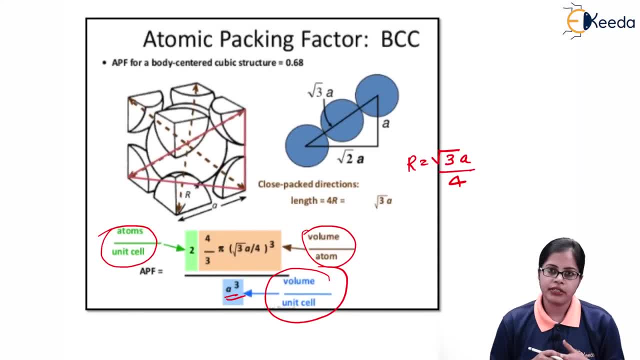 And when we talk about the calculations of body centered cubic unit cell, in this case we are getting the body centered cubic unit structure having atomic packing fraction of around 0.68. so if I 0.68 packing fraction for body centered, so if you want to calculate what is the percentage void? 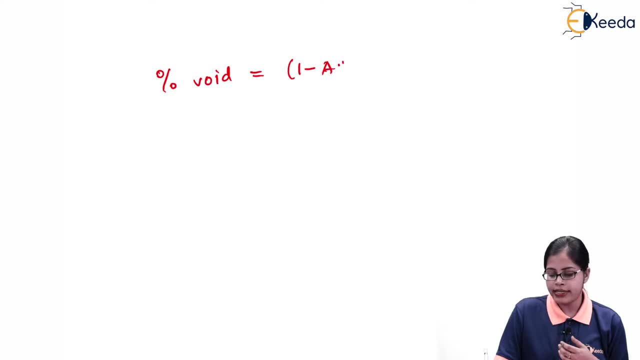 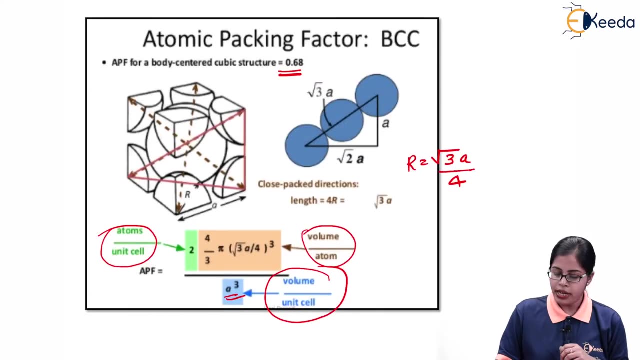 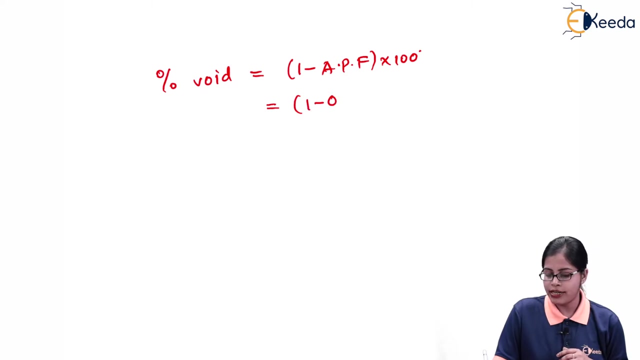 which is present in it. it is going to be taken as 1 minus atomic packing fraction into the 100, because we are calculating the percentage void, as we are aware that the atomic packing fraction for body centered is around 0.68. that is, 1 minus 0.68 is going to give me the value of. 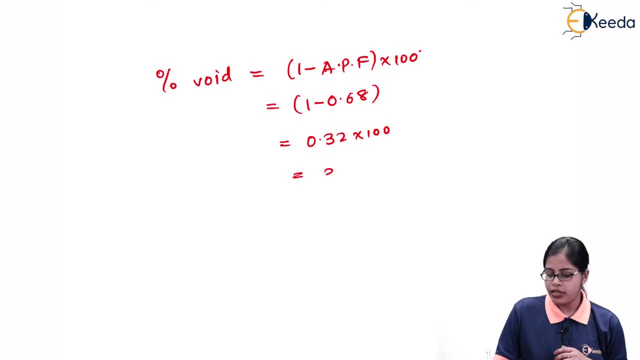 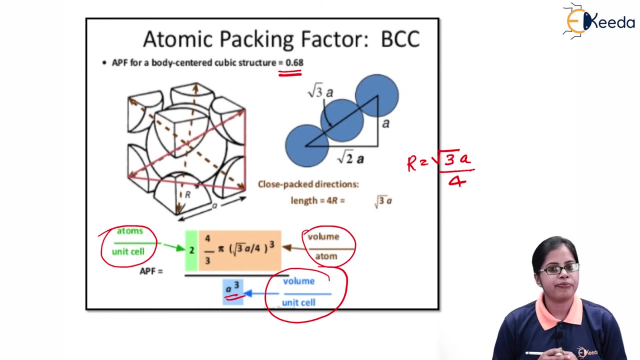 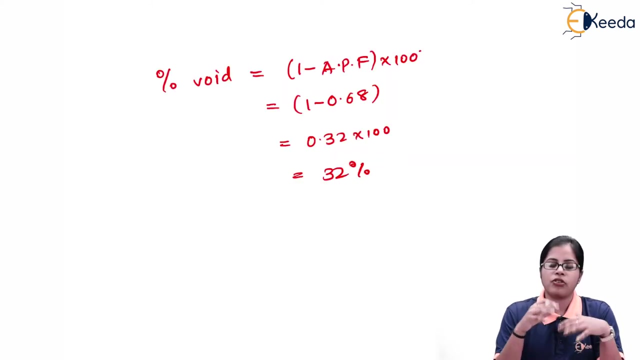 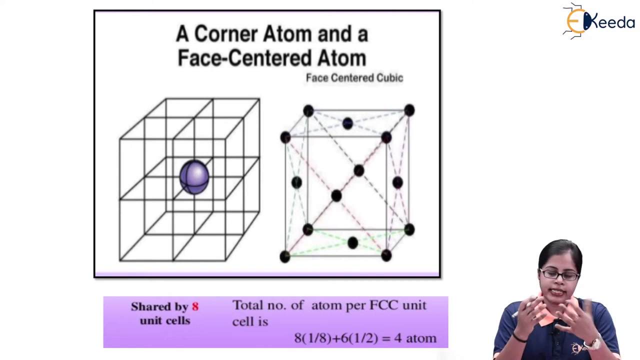 0.32 into 100, that is around 32 percent. so the percentage packed is going to be 68 percent is going to be packed with atom in a bcc unit cell but 32 percent void is going to be present, or 32 space will be present in a body centered unit cell. now, when we talk about the next type of 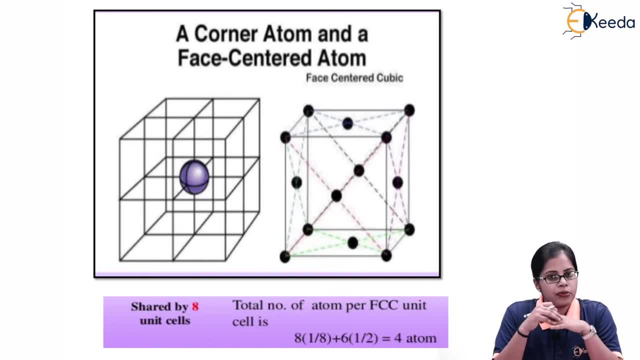 cubic unit cell. as you all remember, we have three types of cubic units: are a simple cubic or primitive. second, we have body centered, which we have discussed just now. and third is face centered. now, if you look at, what do you mean by face centered? is that we are going to have 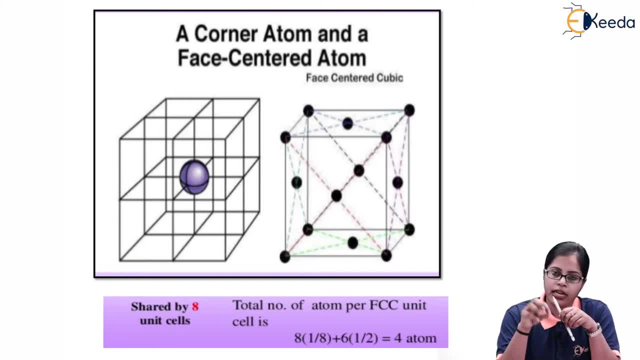 8 corners of the cubes. so 8 lattice points are going to be be attached at the eight corners. then we are going to have one at the each faces of the cubic unit cell. so that means we can say that how many faces are present for the cube? obviously there are six. 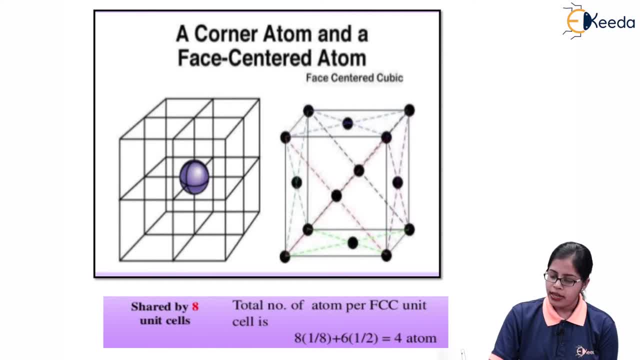 faces of the cube. so we can say over here: is that like when you talk about one, two, three, four, five, six, seven, eight? this indicates eight lattice points at the eight corners of the face centered cubic unit cell. then one for the upper face, one for the side face, that is right face, one for the. 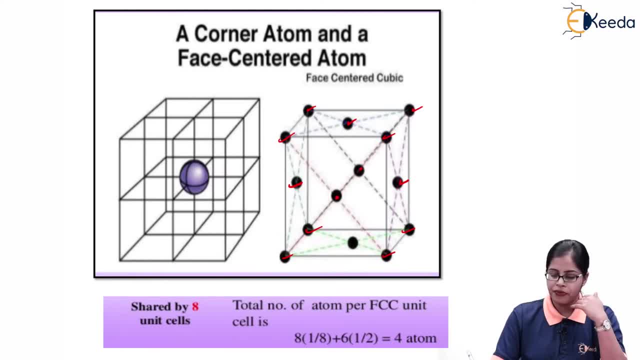 left face, then one for the front face, one for the back face and one for the bottom. so for the faces, has cube consist of six faces so we can have six atoms each face. so that means you can have six atoms per face. so when we are talking about the face centered cubic unit cell, the cubes consist of six faces and if i have six, 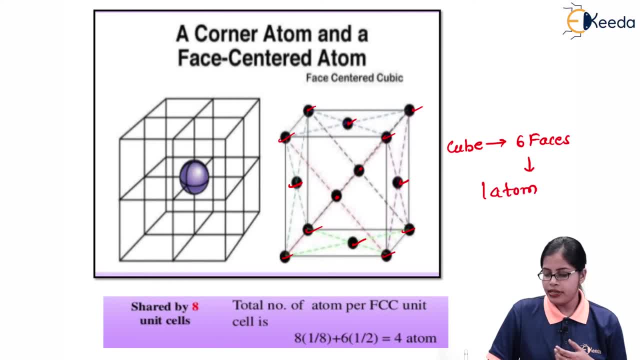 faces. that means one atom present per face. that means we can have six atoms overall for all the faces. next is when you talk about the number of whole atoms which are present for the face centered cubic unit cell. for the corners we can have make use of the same. 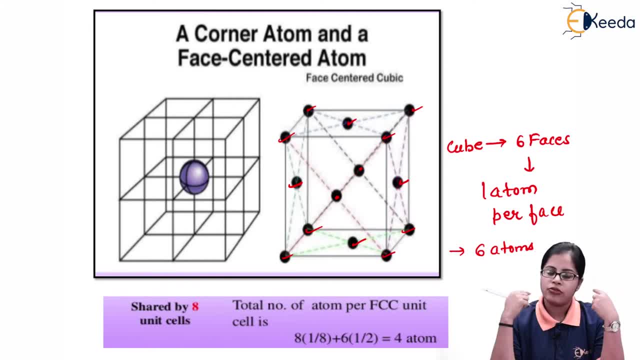 analog, that is, that one atom is getting linked to the eight neighboring cells. so one atom, one eighth content is going to be contributed to each unit cell. so this is the one which is contributed to by the corners or by the lattice points which are available at the corners. and, as we are aware, 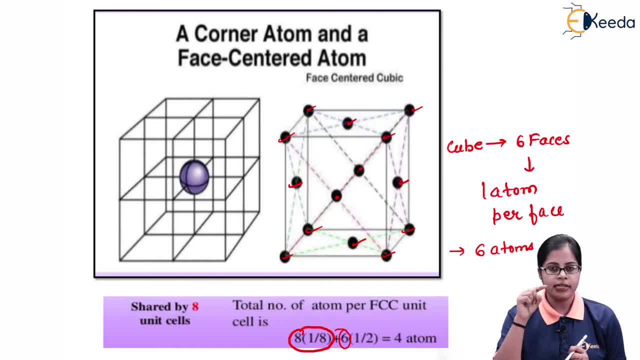 that the six is going to be present at each faces. like i have one atom present at each face of the unit cell, so for one face we have one atom. so this one atom will be linked with two unit cells that are placed beside each other, so we can say the atoms which are present at 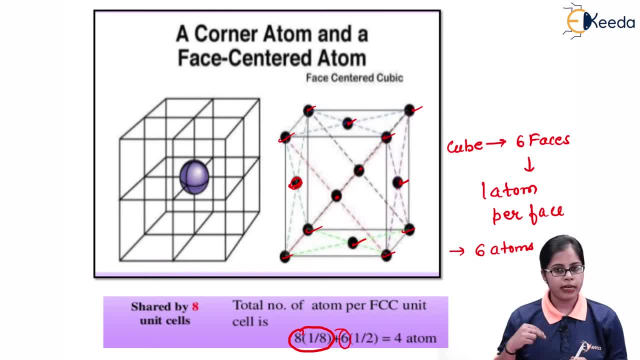 all the six faces will be linked with two neighboring unit cells, one of one and the other one, the one which is neighboring one. so for the eight corners, one. they are contributed one eighth time as they are linked to eight unit cells and the atoms which are present at the six 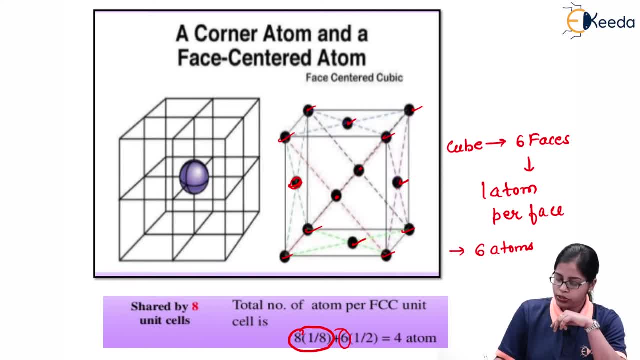 faces are linked to two unit cells, so 6 is going to be contributed 1 by 2 times. so if I overall calculate the value this is going to give me, the value has 1 and this is going to give me the value has 3. so the total overall number of atoms which are present per unit cell. 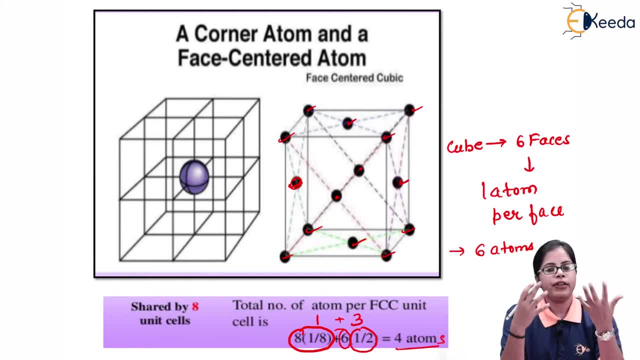 is going to be 4 atoms. so if we can want to calculate the number of atoms which are present per FCC unit cell, it is going to be the one atom for the corners one and the three atoms for the face one, so the overall number of atoms per unit. 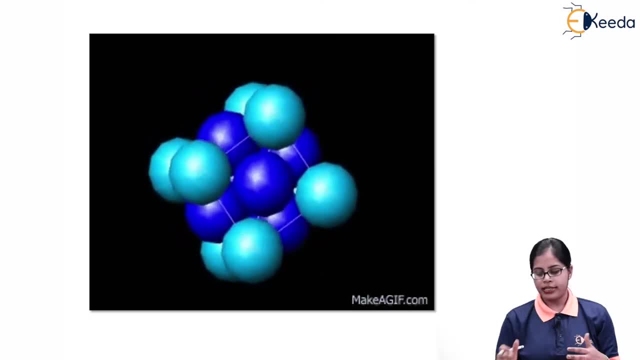 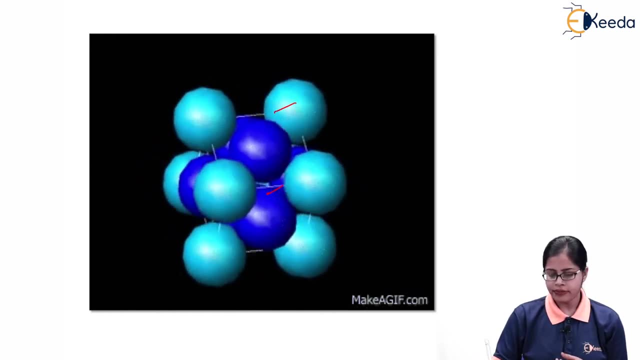 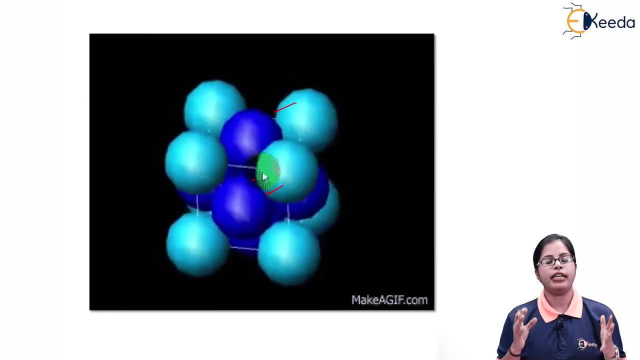 cell of the FCC structure is going to be four atoms. this is how the FCC atoms look like. like this light blue color one indicate the atoms which are present at the corners and the dark blue ones indicate the atoms which are present at each faces. this diagram is only indicating for one. 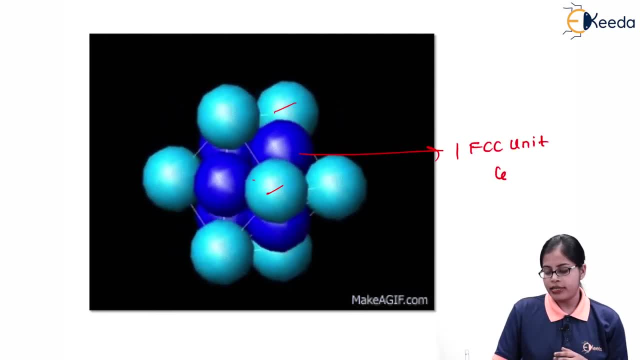 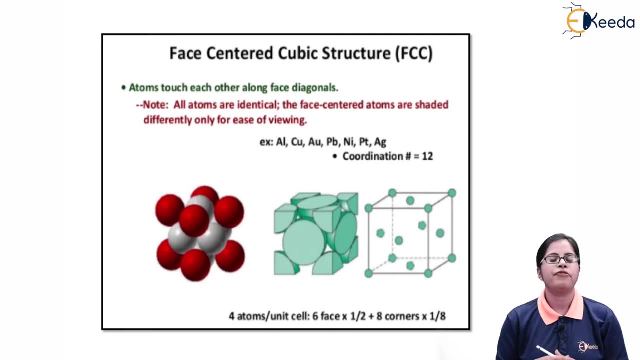 FCC unit set in a similar manner, we can stack all the FCC unit cells together and we are going to make use of, or we are going to get a formation of FCC crystal structure. now again, in this case, when you talk about the FCC structure, the atoms are going to touch each other along the phase diagram. 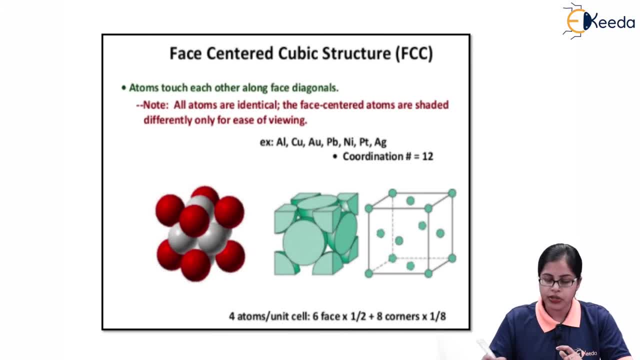 that is not along the cube diagonal. they are going to touch along the phase diagonal. secondly, as you can see in the diagram, we have represented atoms by different shapes of color, but they are all representing identical atoms. we have just made use of different shapes because the red ones are indicating the 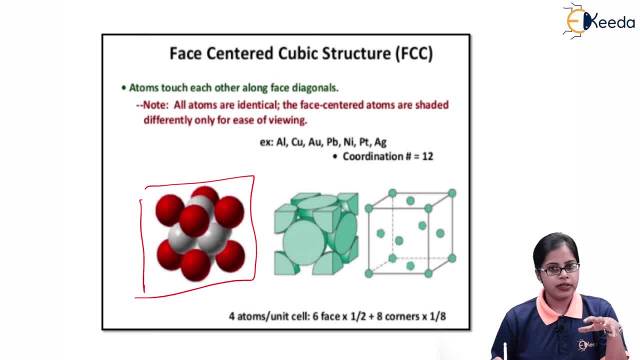 atoms which are present at the corners and the silver ones are indicating the atoms which are present at each faces, faces of the cube. so this different shades of the fcc structure is just used for the different atoms present at different location. this is how you talk about the formation of fcc, that is face. 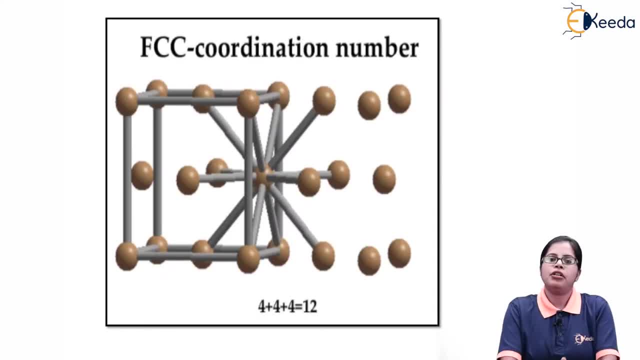 centered cubic structure. now the question comes that what is the coordination number of fcc structure? so if you want to calculate a coordination number, we need to get to know that what is the number of nearest neighbor present to the central atom? so if i consider this as the central atom, the one atom present over here is considered to be the central atom. 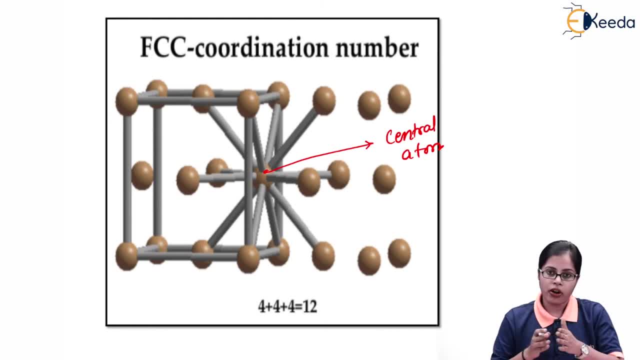 the one central atom is considered or surrounded by one, two, three, four neighbors on this side, one, two, three, four neighbors up and below, one, two, three, four on the left hand side. so the central atom is attached to four neighbors on the right, four neighbors on the left and the four two up and two down, so the total number of nearest neighbor to 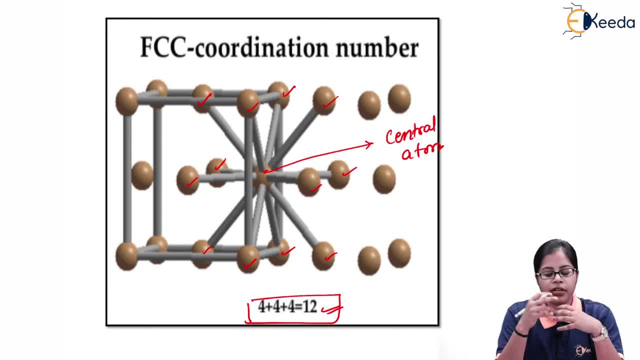 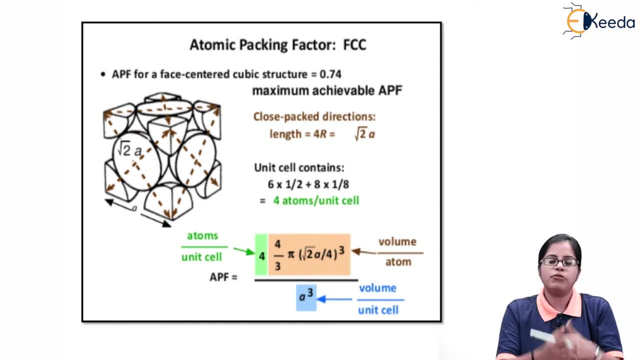 the central atom is going to be 12.. so the fcc coordination number is considered to be 12.. next, if you want to calculate that how much part of the fcc structure is filled with atoms or how much part is packed with atoms, that is, if you want to calculate the atomic packing fraction, 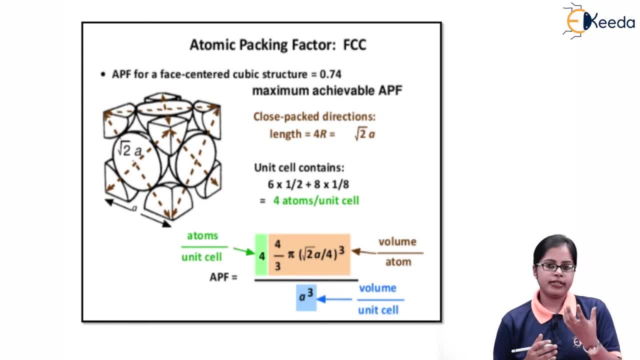 here we're going to make use of again the same formula, that is, the atoms per unit cell into the volume of each atom divided by the volume of unit cell. if i get to calculate the values, this is obviously giving me the value that is, 4 by 3 by r cube, where r is indicating the radius. 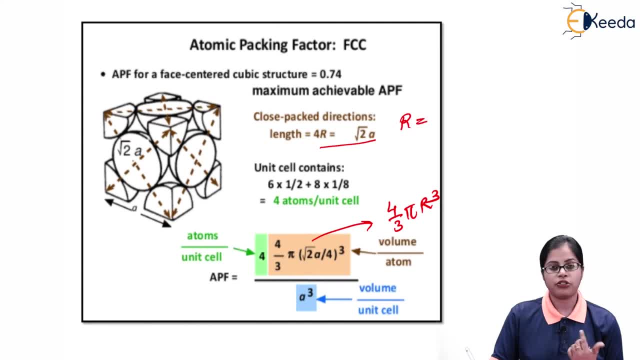 of atom, as we get the radius in fcc structure to be around root 2a by 4, and we can calculate this radius using the help of this diagram. so, if i get to know that, what is the volume of each atom that is using this parameter? as we are aware, the number of atoms 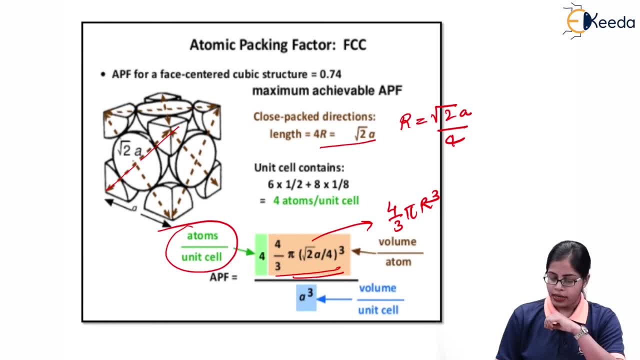 are present. per unit cell of FCC structure is 4 divided by the a cube. if I keep on calculating the whole value, their atomic packing fraction of face centered cubic structure is around 0.74. that means out of all the three material or out of all the three types of cubic unit cell, that is simple body centered. 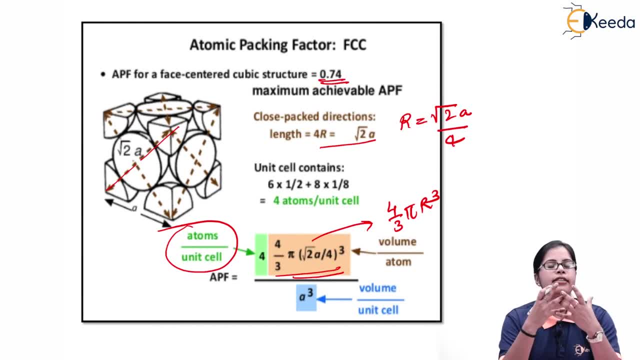 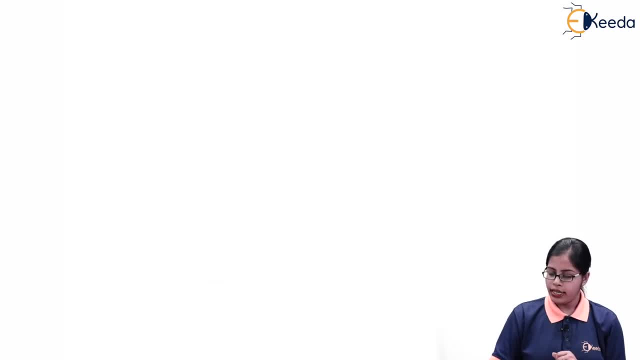 and face centered. the one which has the highest atomic packing fraction is the face centered one because of the arrangement of atoms in that and obviously, if you want to calculate the percentage void in FCC, it is going to be 1 minus atomic packing fraction in 200 and, as we are aware, 1 minus atomic. 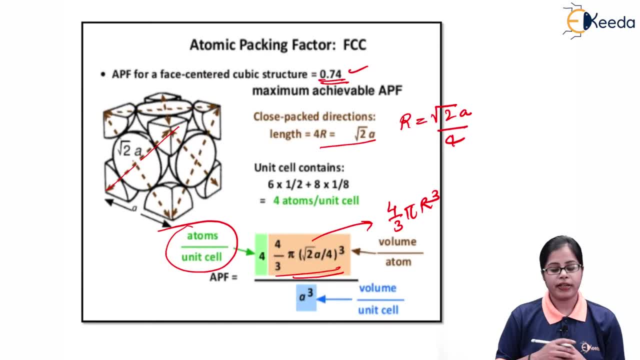 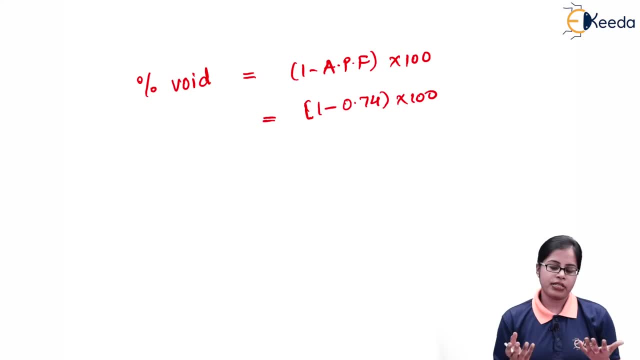 packing fraction. the atomic packing fraction of FCC is 0.7 force, so it is 1 minus 0.7 for in 200, and if we obviously calculate the value of this over here, we are going to get around 0.26 and 200, that is around 26. 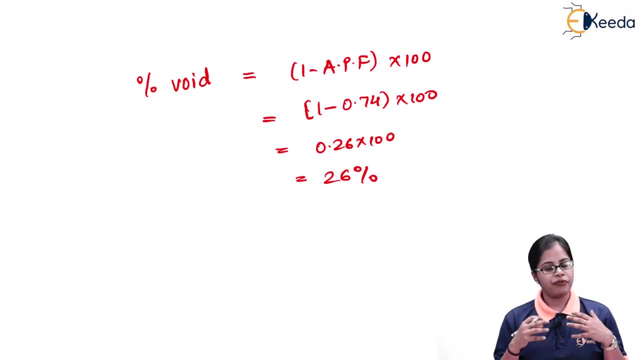 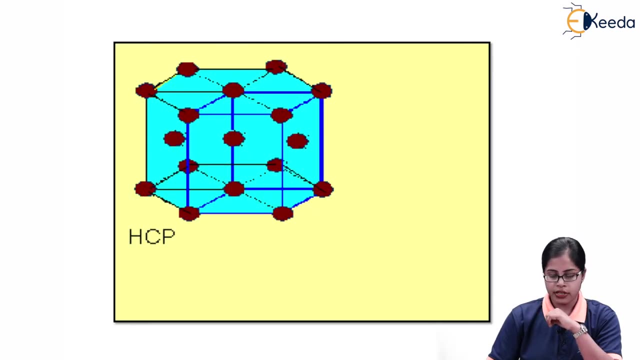 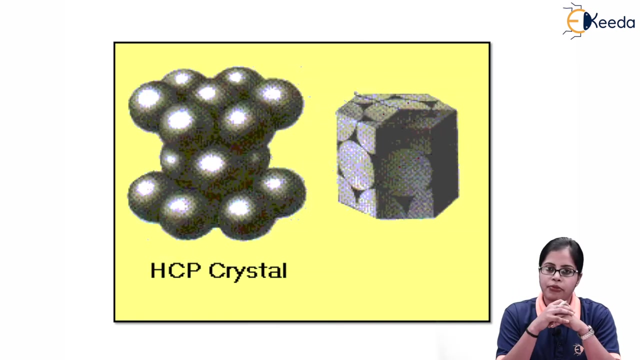 percentage void in FCC structure. so we can refer from this three concepts is that we have minimum percentage of void in FCC unit cell has compared to the remaining unit cells. that is simple, cubic or primitive and the body centered. this is next when we talk about the next type. 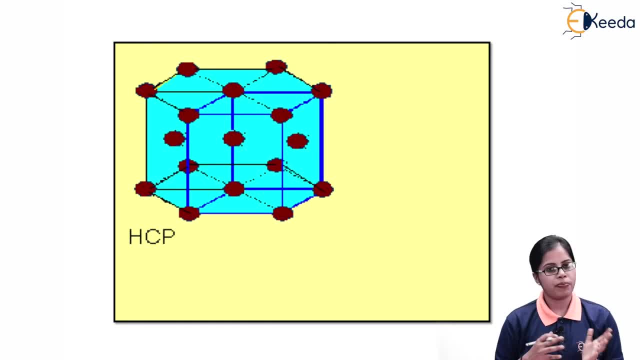 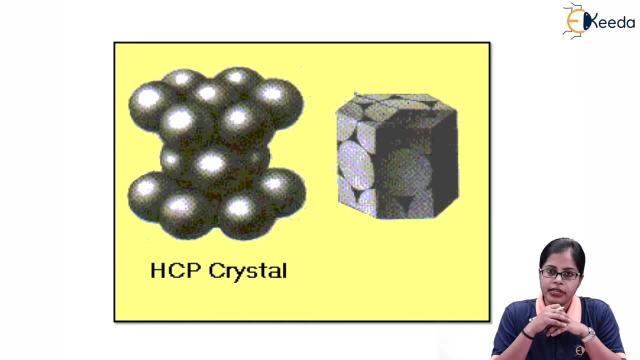 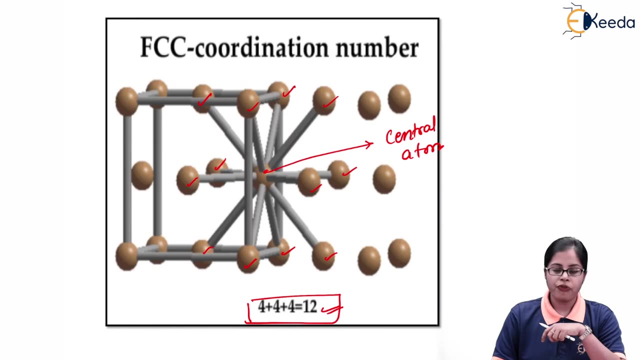 of crystal as hexagonal closed-packed crystal. so till now we were talking about basically the types of cubic units in. when you talk about the hexagonal closed-packs structure, this was that one type of crystal packing you have, or you can say this was the one type of. 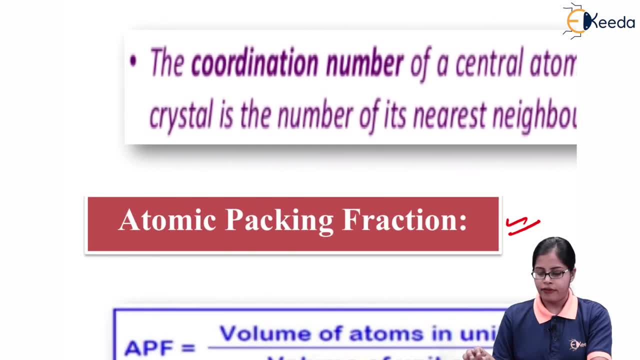 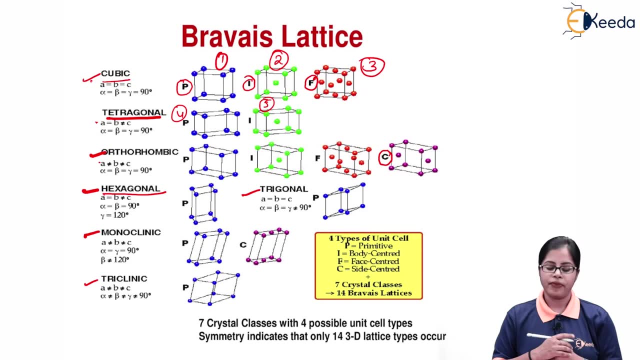 crystal system we have. in this case, like when we talked about the brevis lattice, the one brevis lattice which we had is the hexagonal, so we have ultimately talked about cubic unit, sin. next we are talking about hexagonal. in hexagonal you have actual length of, not equal length, because we get. 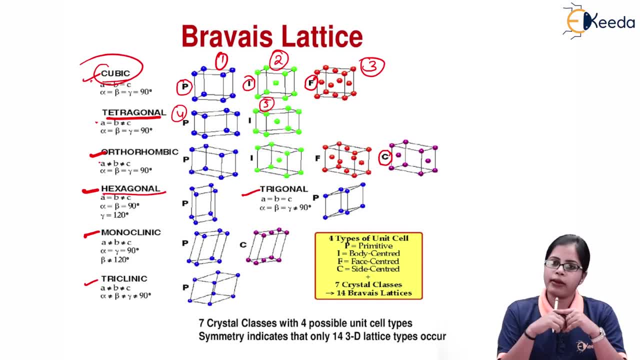 to know that we have two equal length, but the third one is not matching with the value, so we have unequal actual length. secondly, the two are interactual angles. in the hexagonal packing is of 90 degree and the one interactual angle is around 120 degree. that means when we talk about the 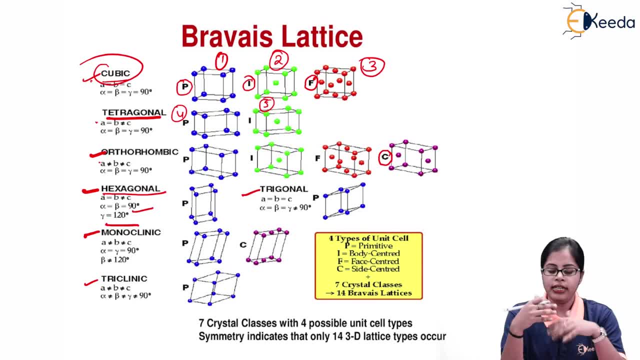 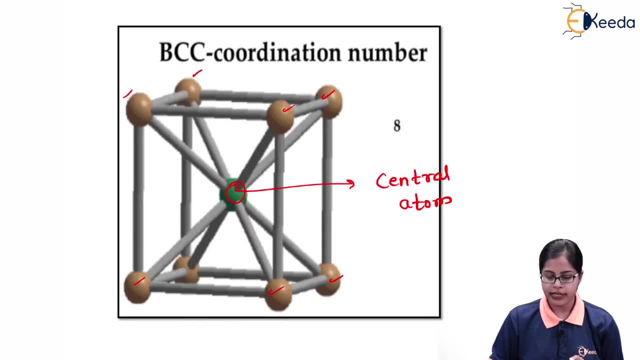 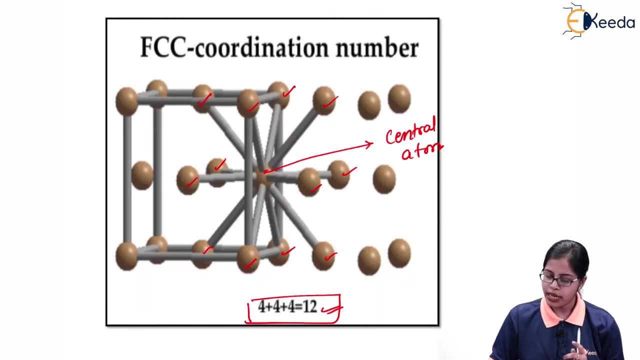 axial length and interactual angle for hexagonal is obviously different from the cubic one. so the structure which we are going to get year for hexagonal closed pack is going to be that is, two axial length to be same and the third one is not matching, and the interaxial angles of two is going to be 90 degree and the third one is 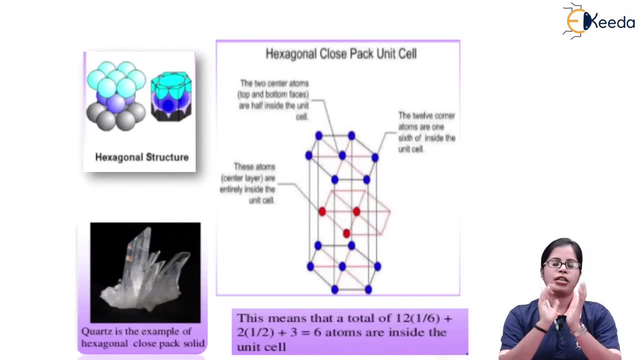 going to have an interaxial angle of 120 degree. if this type of lattice parameters are given to you, the structure which we are going to get is a hexagonal closed pack structure. now, how does a hexagonal closed pack unit cell looks like? now, if you look at the diagram, we have two center. 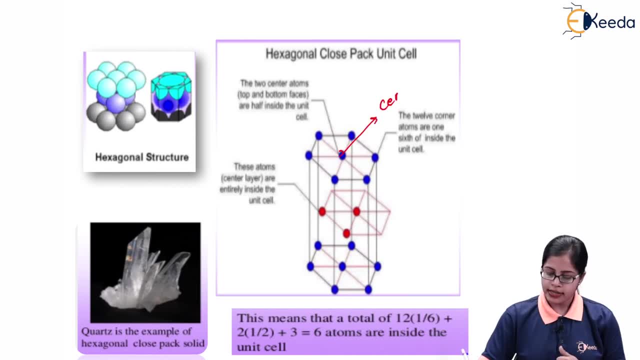 atoms, that is one- this this is indicated as the center atom- and one at the bottom. so we have two center atom, one at the top and one at the bottom, and they are supposed to lie half inside the unit cell. they are not completely inside the unit cell. 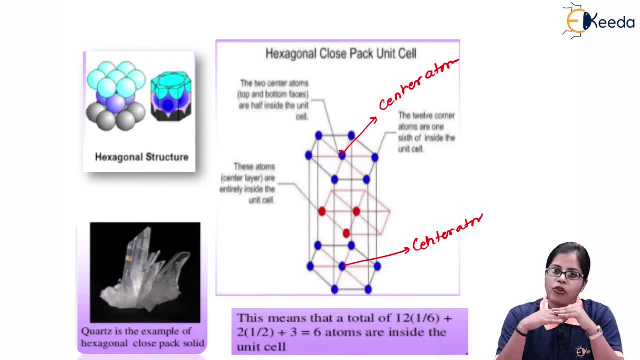 that means two center atoms, one at the top and one at the bottom. they both are lying half inside the unit cell. so next is the three atoms which are present at the center layer, that is one, two and three. they are present entirely inside the unit cell. that is the center layer having three atoms all. 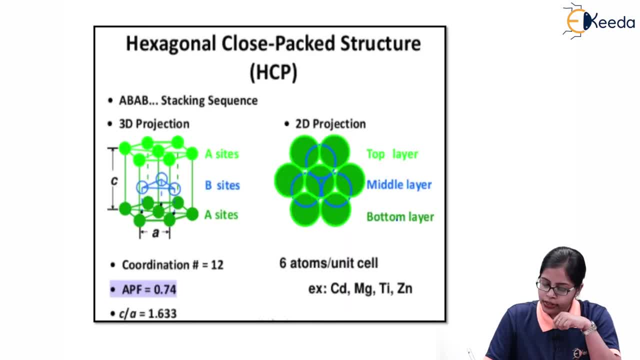 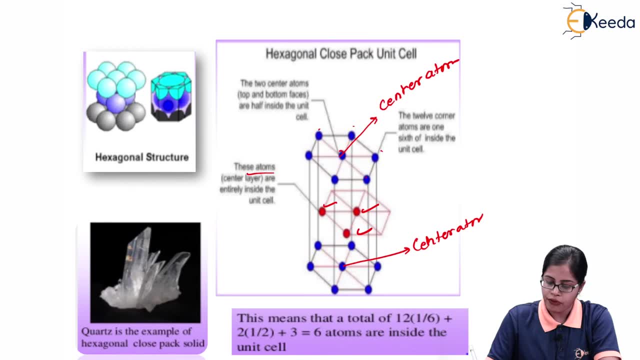 the three atoms are entirely inside the cell. next is, if you talk about the atoms which are present at the 12 corners, that is one, two, three, four, five, six, six at the top layer, one, two, three, four, five, six at the bottom layer. so the whole number of corner atoms, that is 12 corner atoms. 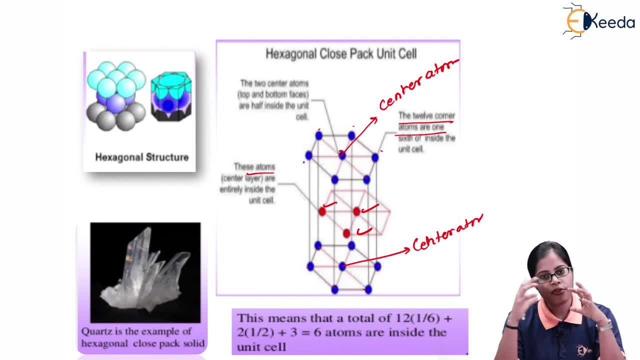 are present. one-sixth of inside the unit cell means they are not even half the one-sixth present inside the unit cell. so if you look at all the atoms that are present inside the unit cell, they atoms the 12th corner. atoms from the six from the top and six from the bottom are present. one sixth. 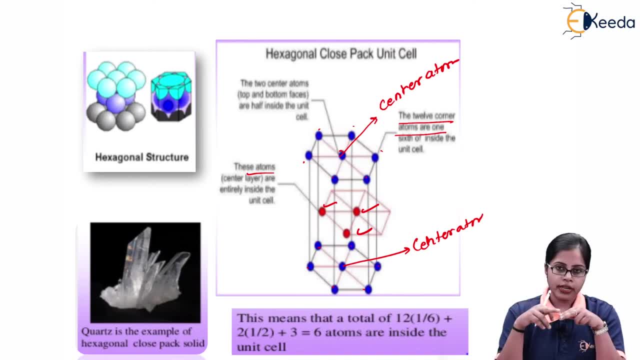 inside the unit cell. the three which are in the central layer, they are completely inside the unit cell, and the two center atom, that is, one at the top and one at the bottom, they are partially inside the unit cells. so if you want to calculate the total number of atoms present inside the 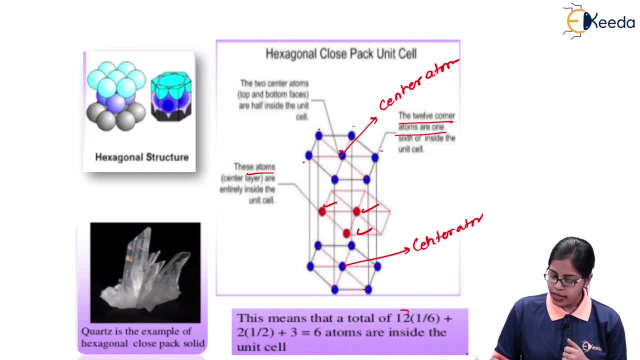 hexagonal closed pack structure in that case has 12 number of atoms, or 12 corner atoms are present, one, sixth inside the unit cell, so 12 of 1 by 6. then two center atoms, that is, one at the top and one at the bottom, is partially inside the unit cell, so it is half of the two atoms. 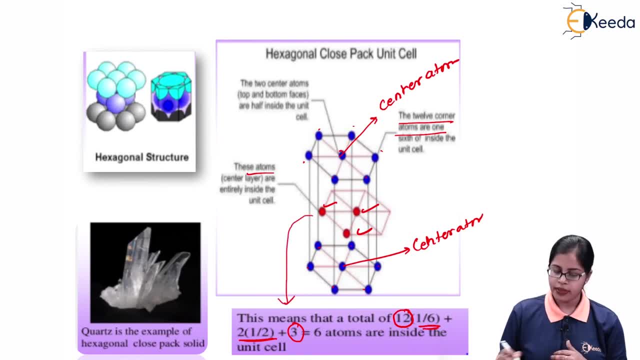 and the three which are present at the center, or the three atoms which are present at the central layer, is completely inside the unit cell. so if i calculate the total value, that is one sixth of 12, one half of two and plus three is going to overall, give me six complete atoms inside the hexagonal closed packed unit cell. 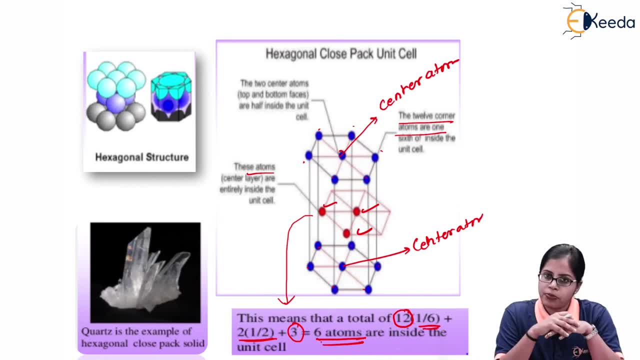 so this is the way we calculate the hexagonal closed pack structure and this is the way we are going to talk about the number of atoms which are present inside the hexagonal closed pack structure. and in real life, the hexagonal structure looks like this, that is, you have a top layer, central. 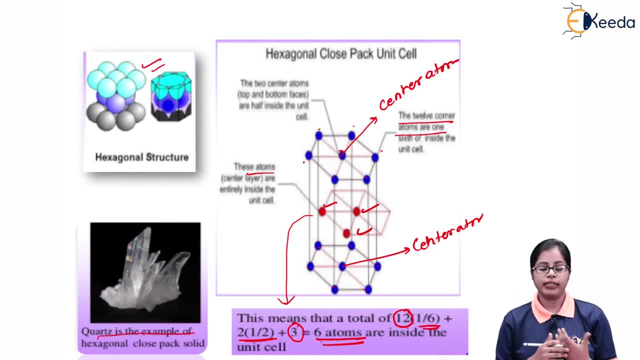 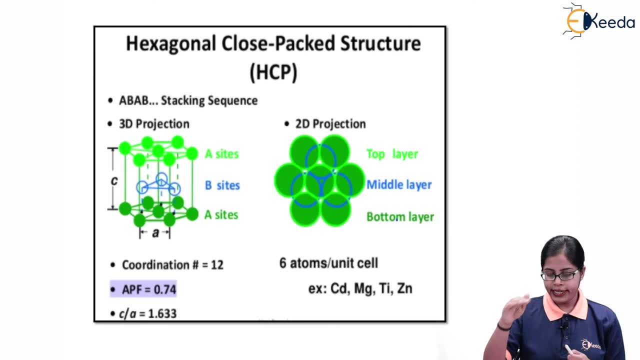 layer and the bottom layer. and quartz is an example of the hexagonal closed pack solid. so this is how the stacking sequence looks like: you have a side, then again you have a b side, that is, a presence of three atoms at the central layer and again you have a site at the bottom. so the stacking sequence is going to be a site, then b side. 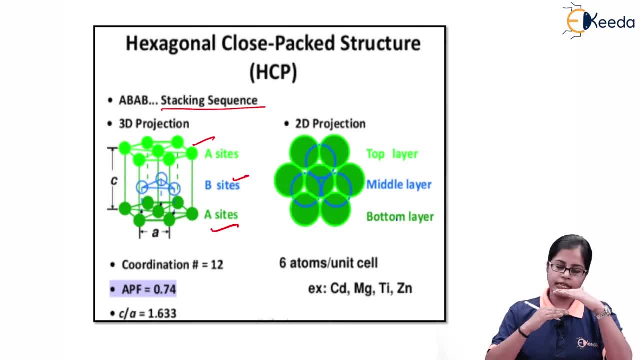 then again we have a side, so you have a top layer, bot middle layer and the bottom layer. as we have calculated just now that there are total number of six atoms present per unit cell for the hexagonal closed pack structure. so this is how the hexagonal closed structure looks like. 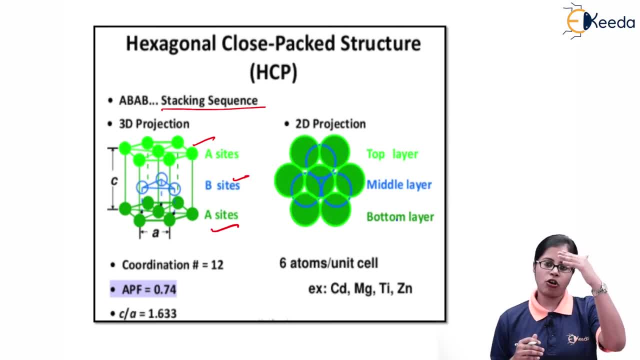 that is abab stacking sequence. you have three layers, that is top, bottom and in between a middle layer and six number of atoms per unit sin. and if you want to calculate the coordination number, in this case it is going to be around one central atom is surrounded by the 12 corner atoms or 12 neighboring atoms. 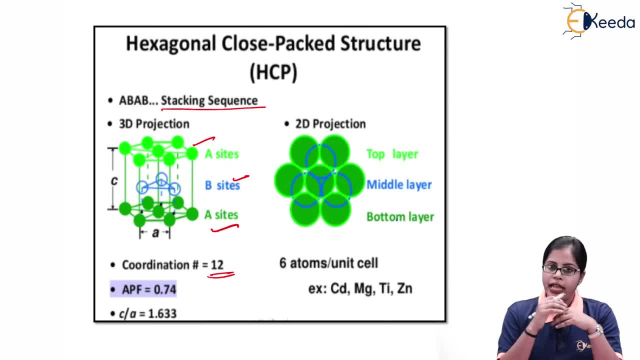 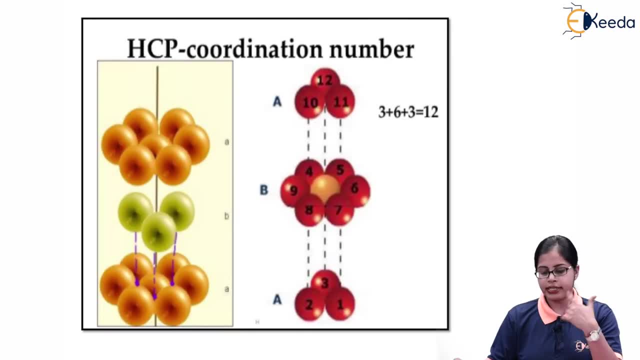 that case the coordination number is given by 12 and the atomic packing fraction for hexagonal is going to be 0.74. and in a similar manner we can keep on calculating the percentage void. and this is how we calculate the coordination number. that, if you look at the central atom, 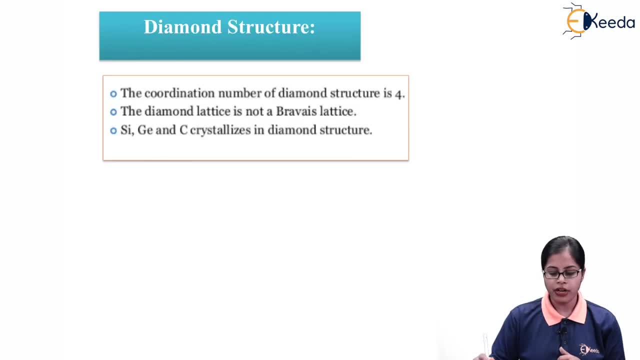 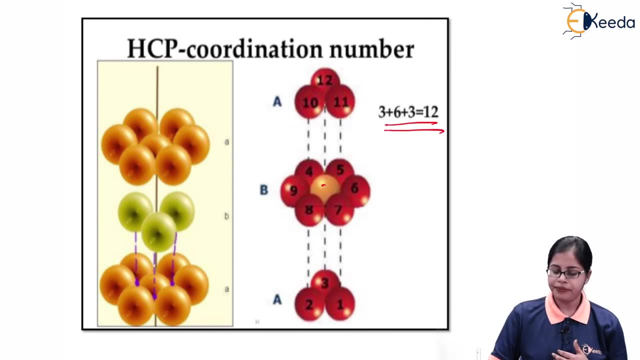 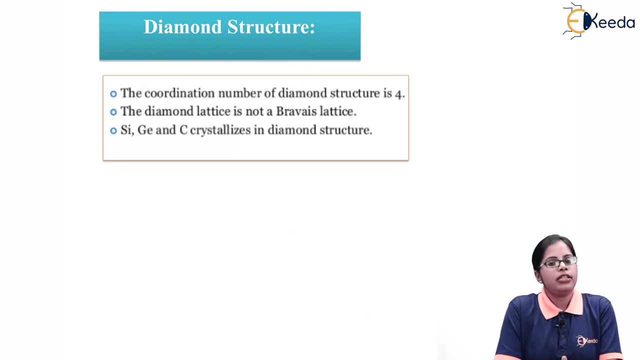 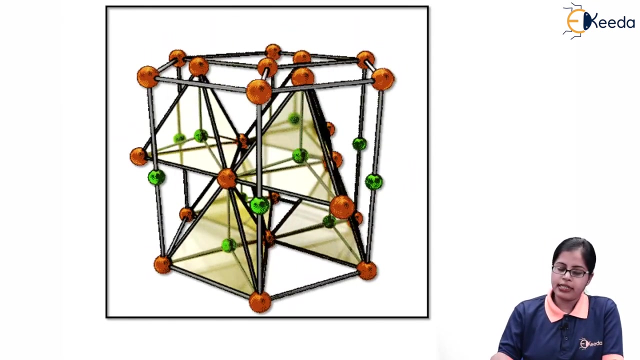 central atom is going to be surrounded by one, two, three, four, six at the center and three, three from top and bottom. so you have total 12. nearest neighbor to the central atom, that is this orange. and the next structure which we require is a diamond structure. as you can look at this particular diagram, this is indicating the structure of diamond. as you can see, 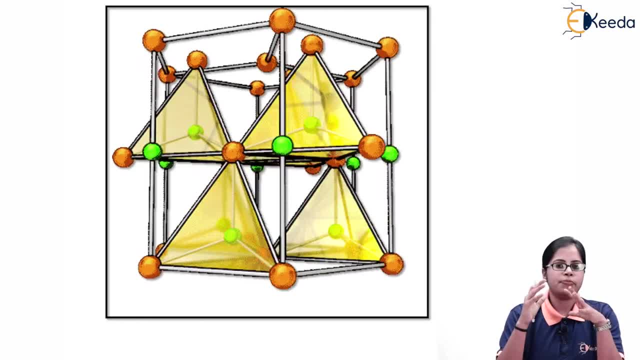 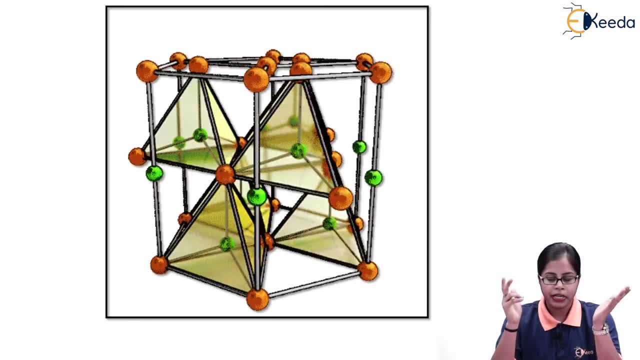 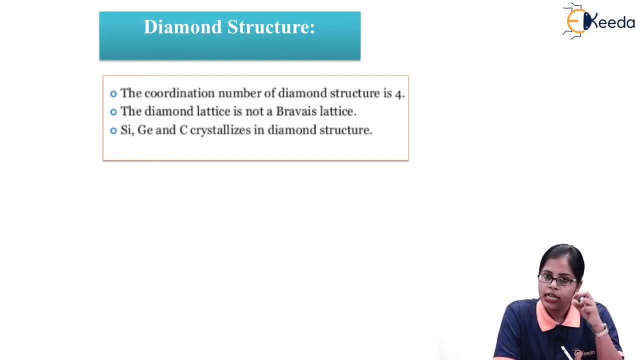 you have the presence of parametrical shape present inside this whole structure, so you don't have one parametrical shape present in it, you have many parametrical shape arranged overall, giving me a diamond structure of crystal and for diamond structure, the central atom of diamonds crystal structure is attached to four nearest neighbors, so hence, 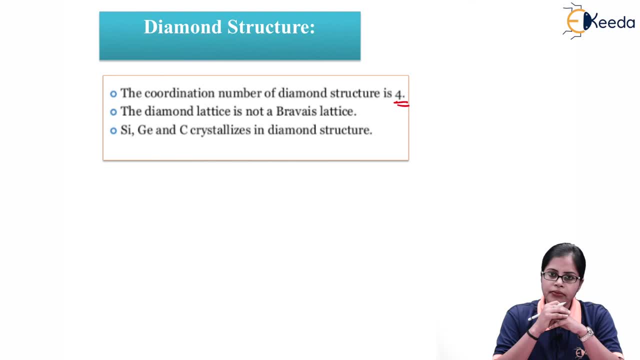 the coordination number is four. second thing: diamond structure or diamond lattice is not to be considered in brevis lattice. and lastly, the examples of silicon, germanium and carbon is considered to be in a diamond structure. so this is what we talk about: diamond structure. this is 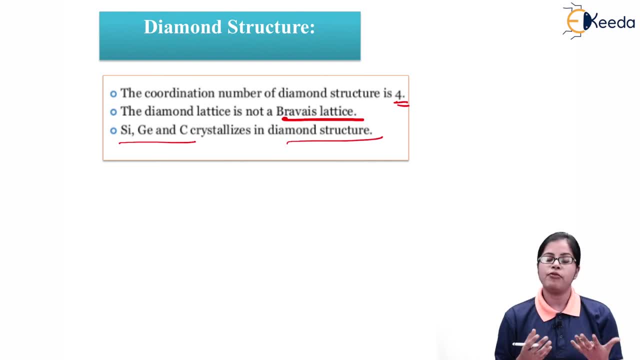 is what we have completely talked about: the basic concepts of crystal structure. how is the there is a formation of crystal structure and the parameters which we use for calculation in the crystal structure. and ultimately, we have even talked about the types of cubic units in hexagonal closed pack and the remaining part of the coordination number and atomic packing fraction. 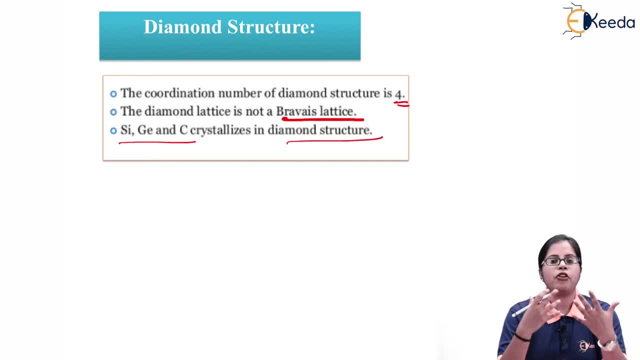 this is the basics which is required for the formations of crystal structure. thank you so much you.